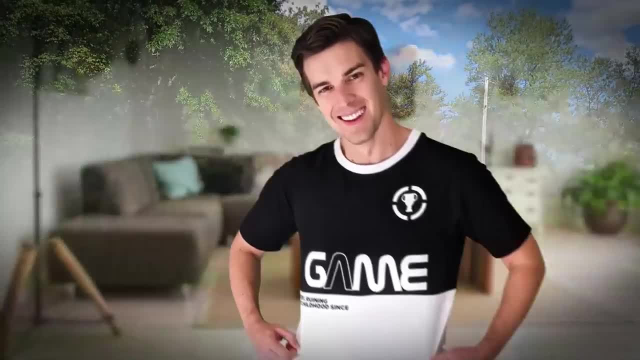 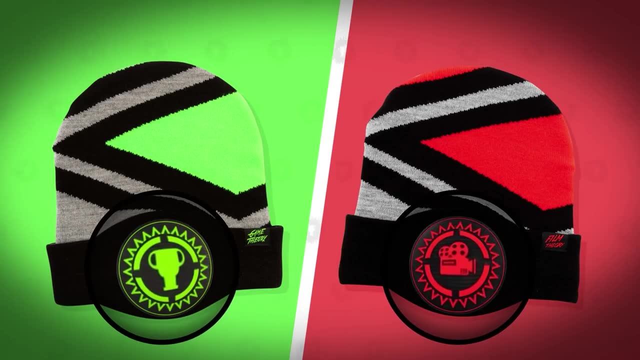 Super comfy while still being super stylish, Whether you're going out chilling around the house or looking to blend in with a chessboard, Need a bit more color in your life. Well, we've got Game and Film Theory beanies with rubber-embossed logos and knitted graphics. 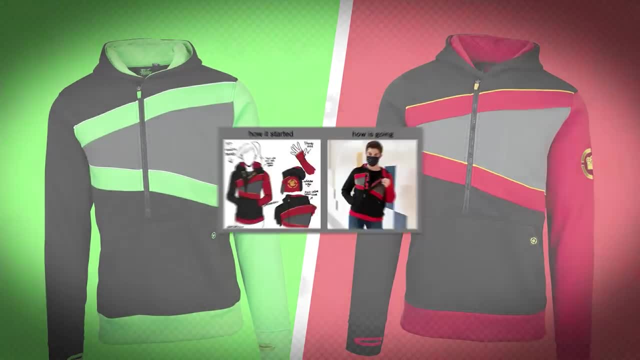 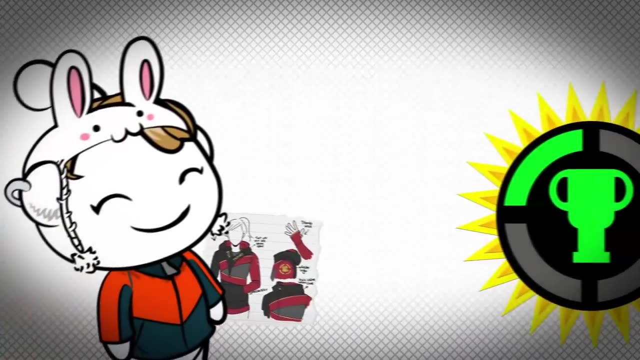 Plus, we've got matching asymmetrical hoodies, The design of which was actually influenced by loyal theorist Sarah. She drew these as fan art and left them on her subreddit. I loved the design so much that we reached out, Purchased the designs and made them into actual clothing. 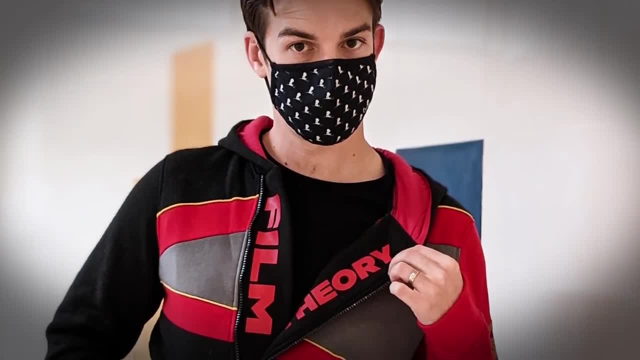 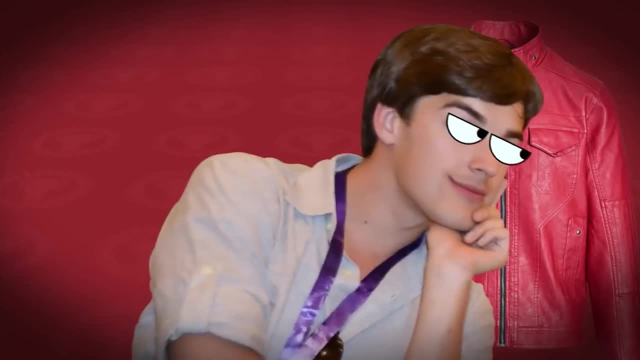 You spoke up, we listened, and now I have myself one of my favorite hoodies to wear in and out of the house. If hoodies aren't your thing, well, we've got two amazing new jackets, Cause y'all know me, if I'm presented with a good jacket, I'm like, yes, all the jackets. 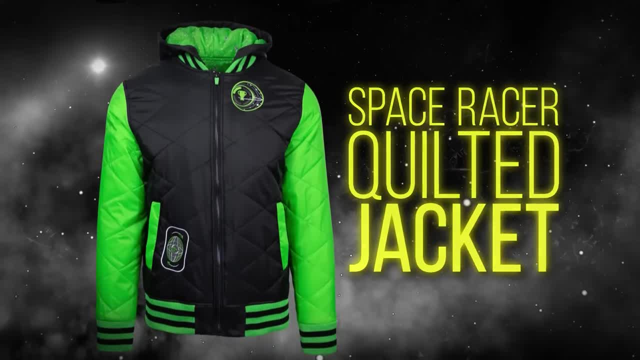 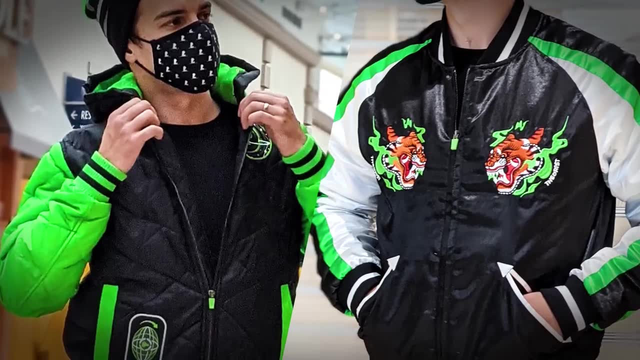 This time we've got ourselves the Outrunner Souvenir Jacket and Space Racer Quilted Jacket. Both are nice and warm and poofy and snuggly And they both have heavy-duty rib-knit cuffs, collars and waistbands to guarantee that they're gonna last for a while. 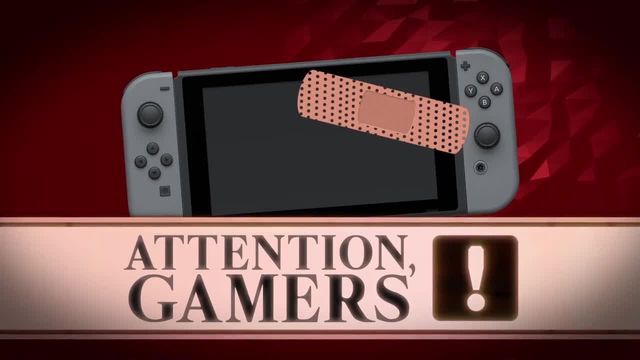 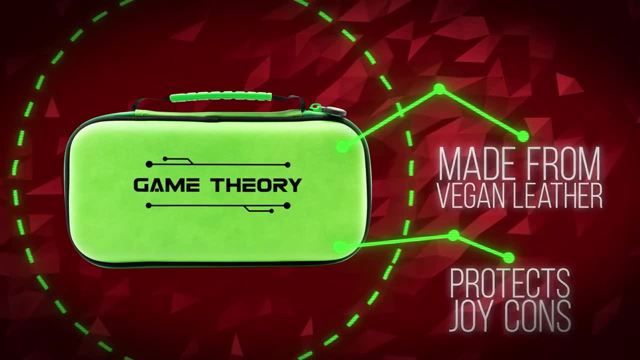 If you got enough clothes- attention gamer. You need to protect your consoles while you're out and about, so why not use our new Alien Tech Switch Case? It's a super durable case made from vegan leather with an interior that's specifically designed to protect your Joy-Con analog sticks. 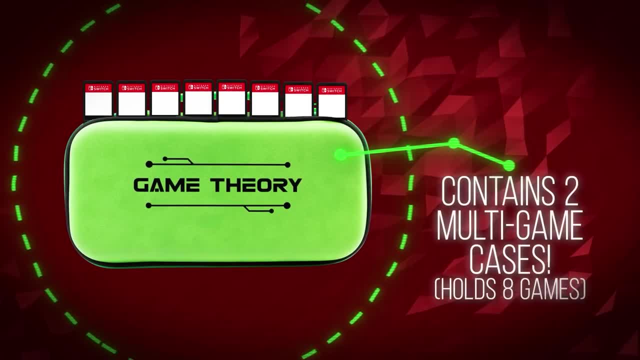 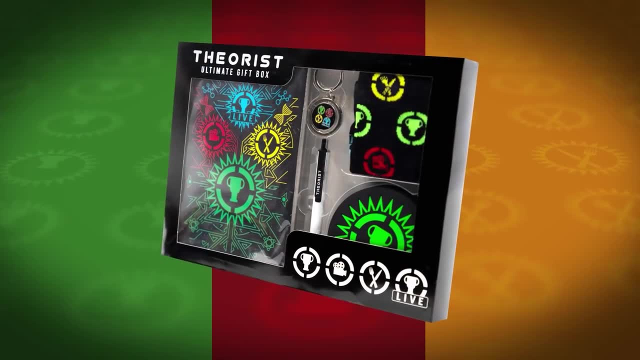 We all know how bad those things can get. Plus, you get two bonus multi-game cases. That is free merch inside of your merch. Maybe you love all our theories and merch but can't decide which is your favorite. Boom, Our four-channel gift box is perfect. 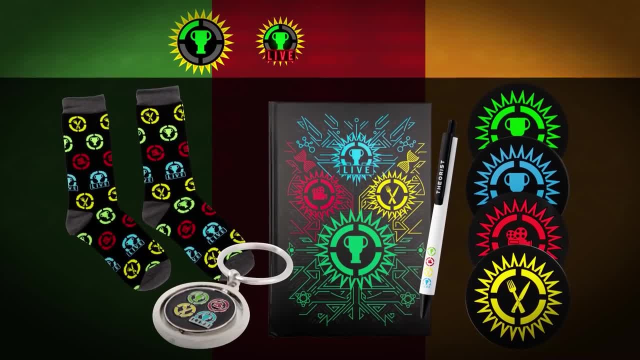 It's got a notebook, pen, coasters, socks and spinner keychain, All sporting the four-channel logos, so you never have to pick your favorite again. Lastly, For all those long holiday nights that you spend cuddled up on the couch, 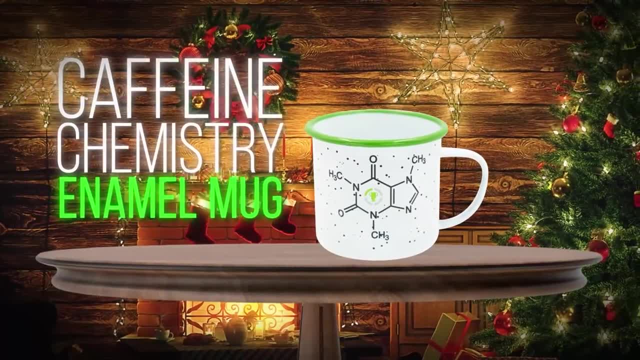 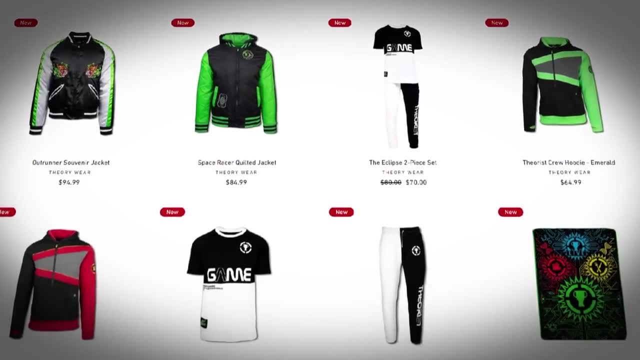 you can enjoy your beverage of choice in our caffeine chemistry enamelware mug, while wrapping up in our super soft, snuggly theories blanket. There is a lot to choose from in this merch drop, but I gotta tell you I adore each and every one of them. 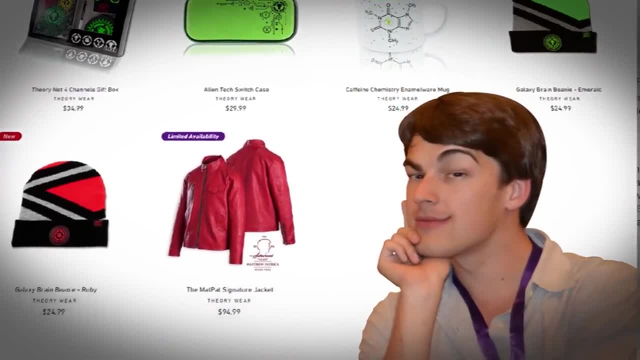 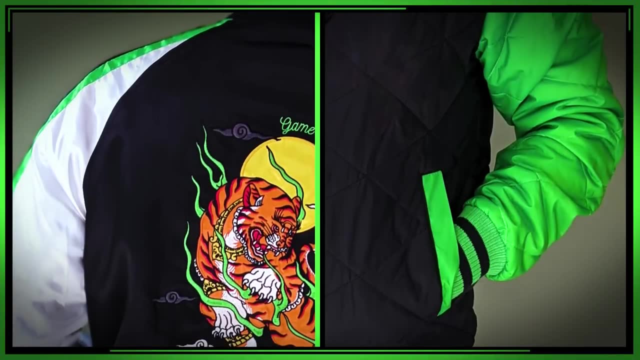 I might have said yes to one too many things this time, but it doesn't matter, As anyone who's ever bought our theory wear can tell you, our merch is in a different league of quality. We only use the highest quality materials and build these things from the ground up because we value you. 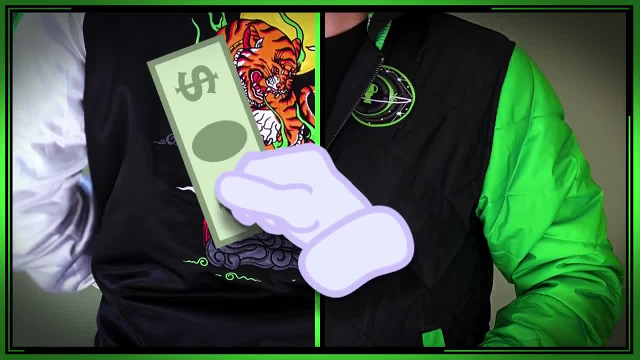 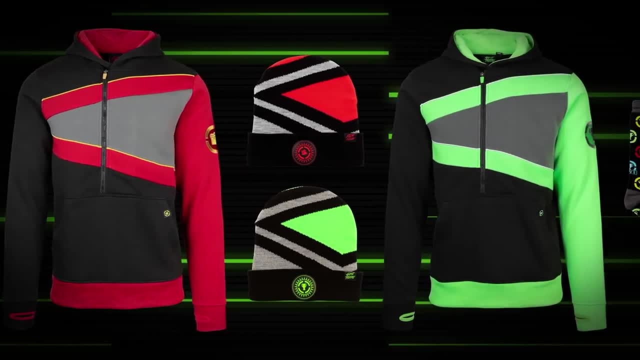 and think that when you buy something, it should actually feel like it's worth it, Something that you're proud of, and not just some logo that's screen-printed onto a shirt. This slate of items is, quite honestly, the best yet, as we continue to learn and find the best people to help build us the best things possible. 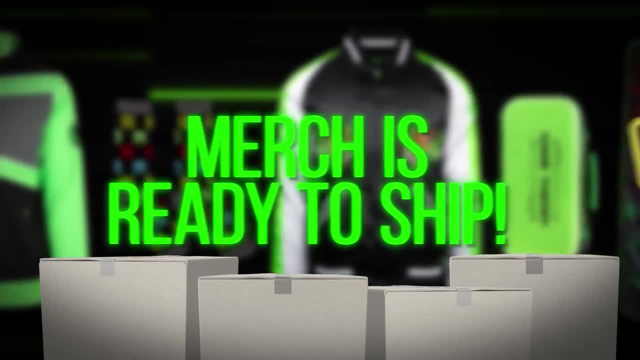 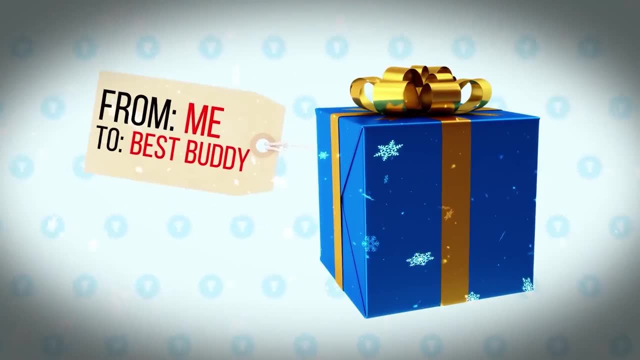 And, best of all, we've already ordered it. It is waiting to be shipped out to you as soon as you place your order, so you don't have to worry about massive delays on it getting to you in time for the holidays. So, whether you're buying it for yourself or fancy getting a gift for some other loyal theorist- 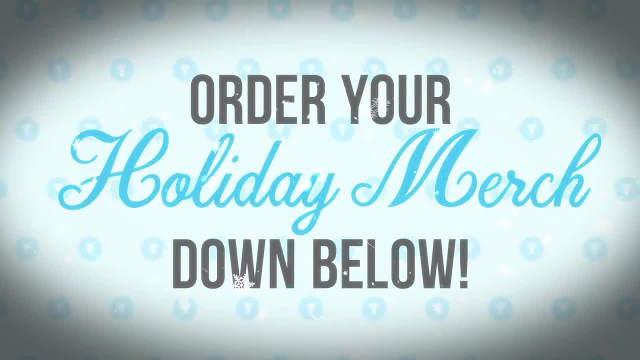 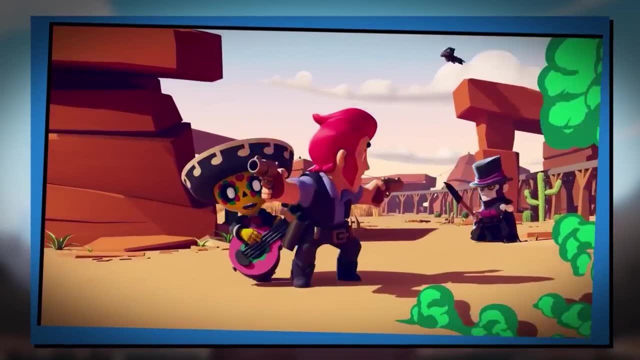 head on down to the description below and snag yourself some awesome theory wear so it can be with you in time for the holidays. And with that shameless plug out of the way, it's time to talk about Brawl Stars. Brawl Stars is a twin-stick hero shooter that's geared towards mobile gamers. 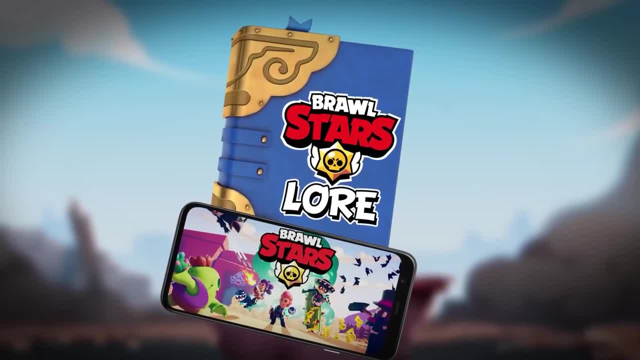 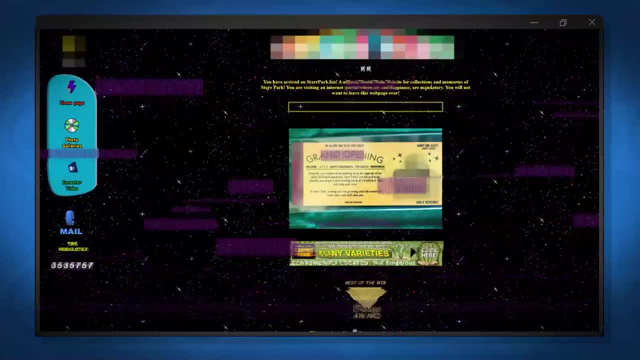 Yeah, you heard that one, right. Not normally the place that you'd expect to find some interesting lore, Unless, of course, you're talking about the weird ad campaigns. So imagine my surprise when I met Kairos at a gaming event and he introduced me to a world full of secret, lore-filled webpages. 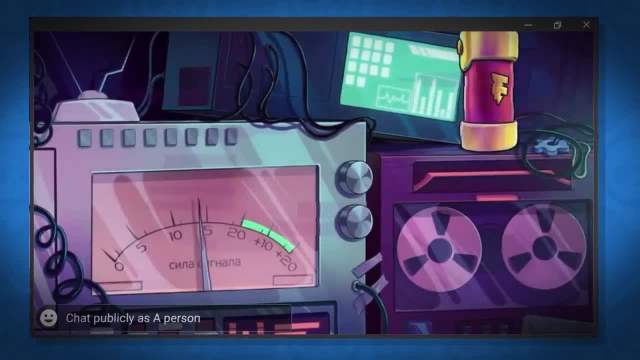 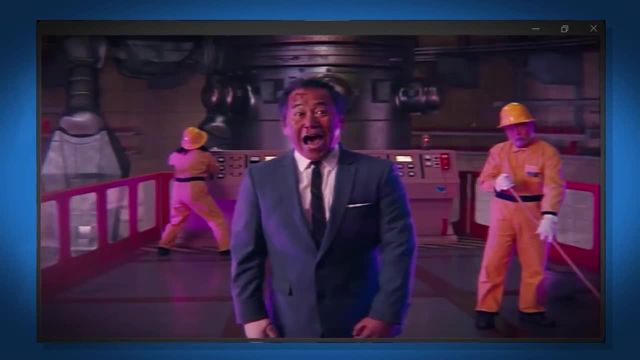 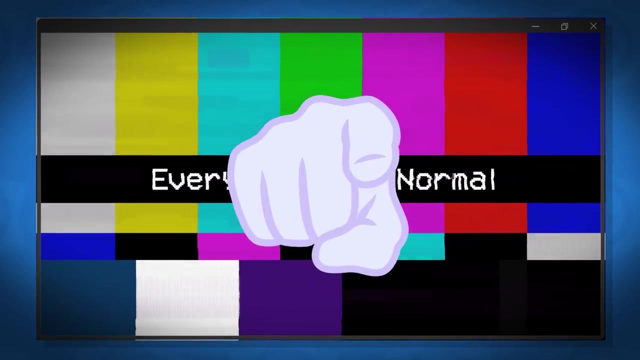 livestream radio broadcasts with hidden Morse code and creepy over-the-top investor videos. Here's a pro tip: Anytime someone tries this hard to convince you that everything's normal, you can be sure that things are anything but, Needless to say, he caught my attention real quick. 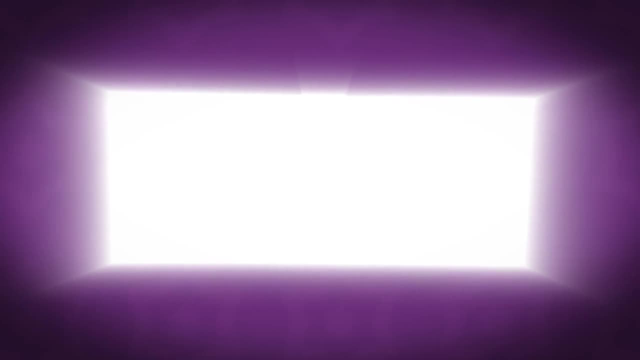 Just kind of wished that I had gotten to it sooner so that I could have been one of the YouTubers to get a secret Star Park package in the mail filled with clues and hints about the game's lore. That's right, ladies and gentlemen. 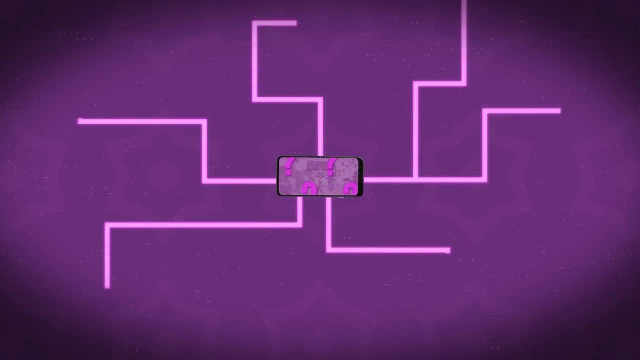 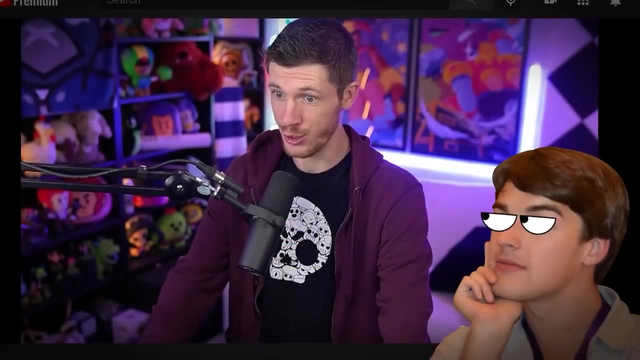 This isn't just limited to the game. This is a fully-blown ARG involving members of the player community. You know who did get one of those Star Park fanpages. You don't have to rub it in. Honestly, you should probably be glad you didn't get a package. 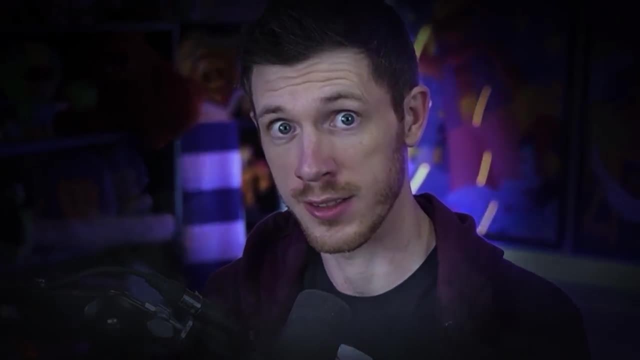 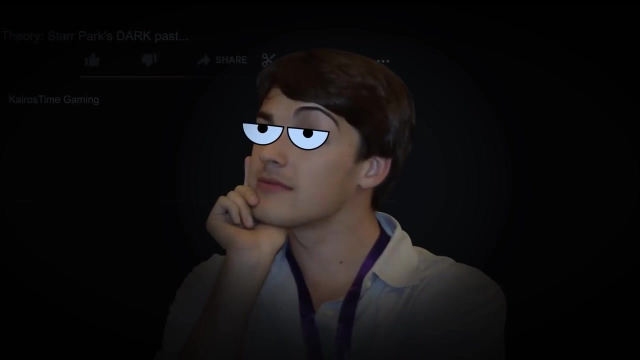 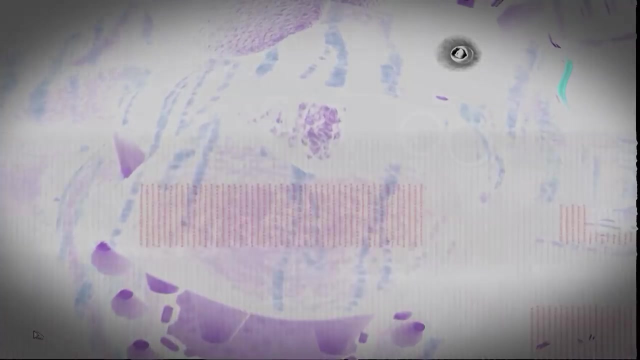 because otherwise you'd have to experience the nightmares that I've been living through every single day. Oh, I know the feeling. I know the feeling. Anyway, Brawl Stars is a game that doesn't present a whole lot of its lore in-game. 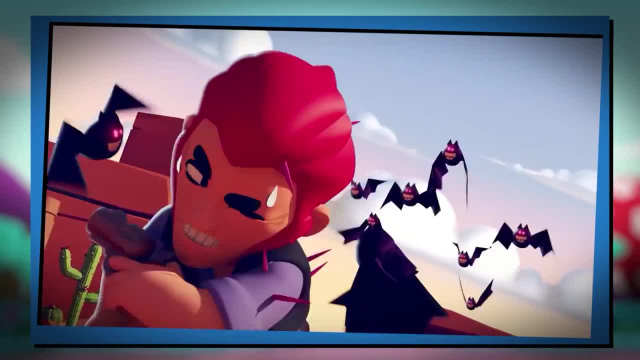 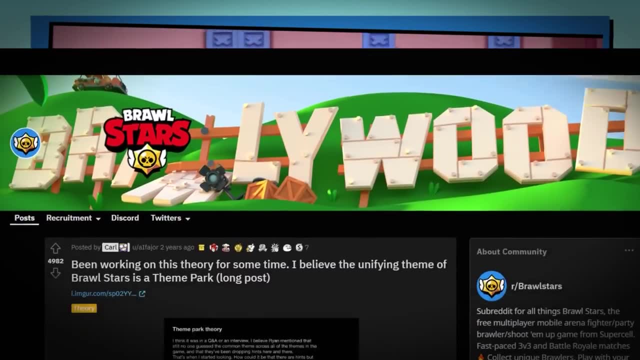 At first it seemed like this was just a game about cute little fighters duking it out to be the first team to collect ten gems or guard a safe from waves of robots, with no reason as to why, Or so we thought. Then came a Reddit post by a user named Gamba. 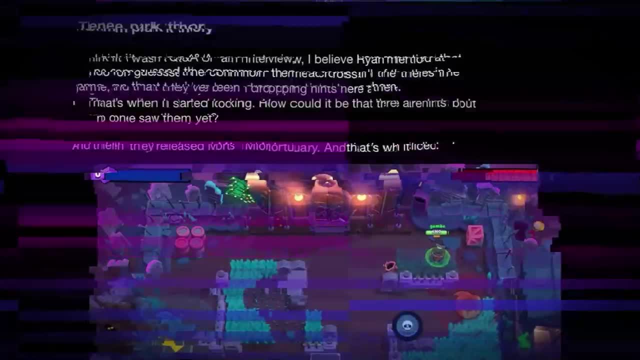 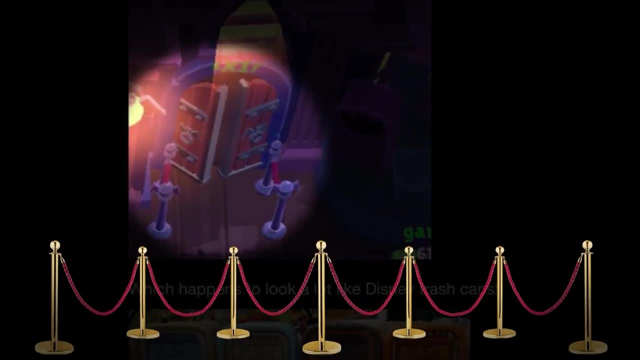 who pointed out that there was something fishy going on with the game's maps. A lot of the fixtures were things that you'd typically find in a theme park. For example, the Mortis Mortuary map has these rope barriers that keep people in theme park lines. 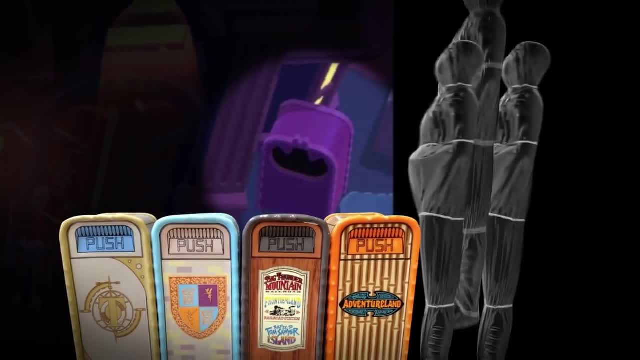 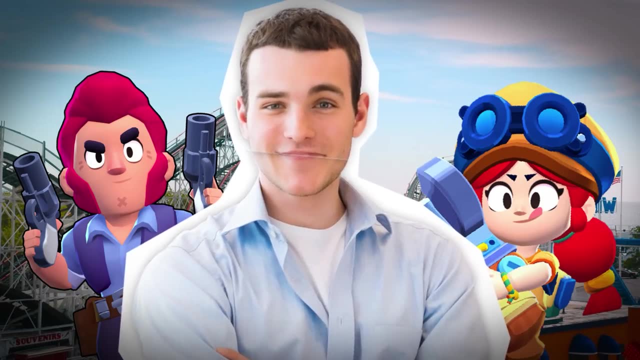 There are also trash cans that would look more at home in a Disneyland than a mortuary. So I hear you saying: the brawlers are all fighting each other in a theme park. That's it. That's the big lore. If only it were that simple, friends. 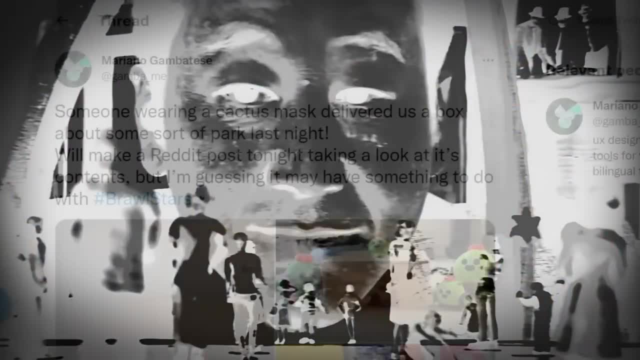 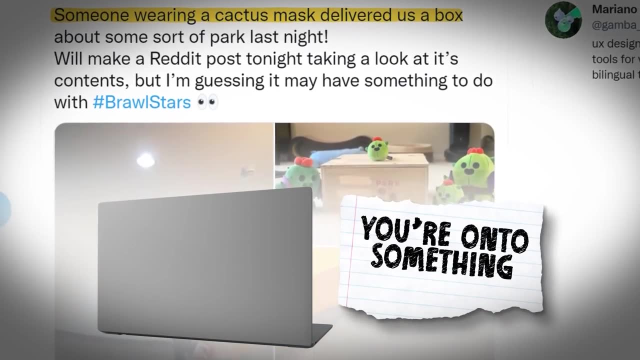 You see, someone was watching and listening. Gamba would receive a mysterious package in the mail later that year containing a laptop and a note saying you're onto something. There was also a link to a website, starparkbiz. Why this mysterious informant decided the best way to send a URL was by hand delivering. 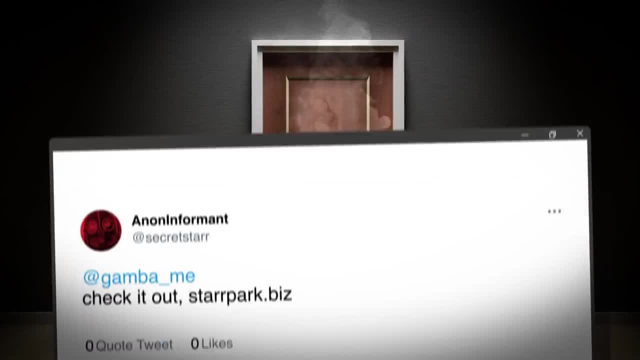 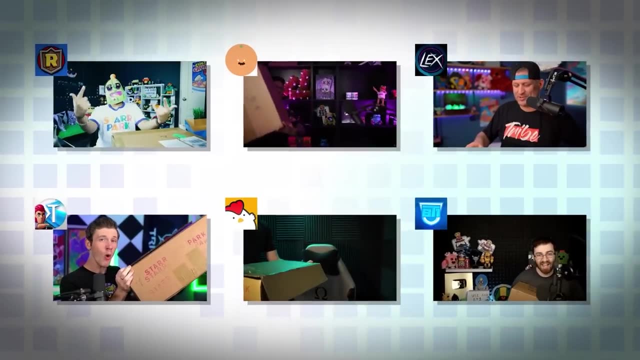 an ancient laptop to their door rather than I don't know, using an internet messaging service is perhaps the biggest mystery of all, And Gamba wasn't the only one. On September 5th, a bunch of community members revealed that they. 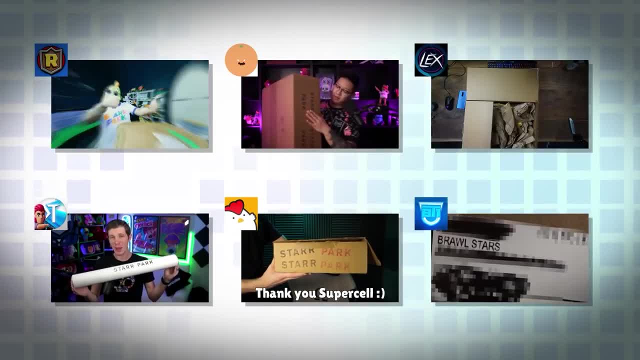 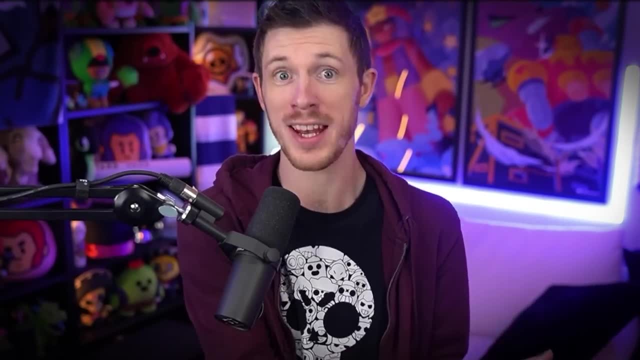 too, had received physical packages full of items from this mysterious Star Park. I'm sorry, but you've got to at least talk about what happened the day before that, where Star Park literally threatened community members trying to get them to stop digging into this mystery. 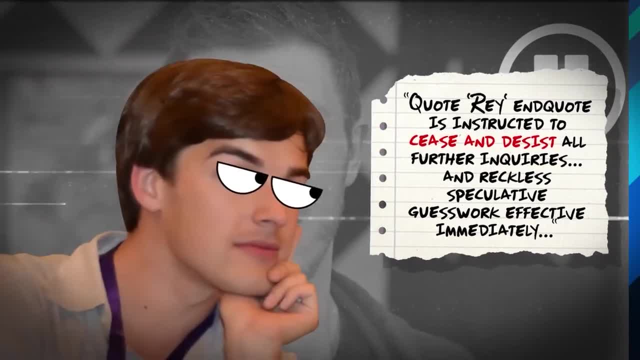 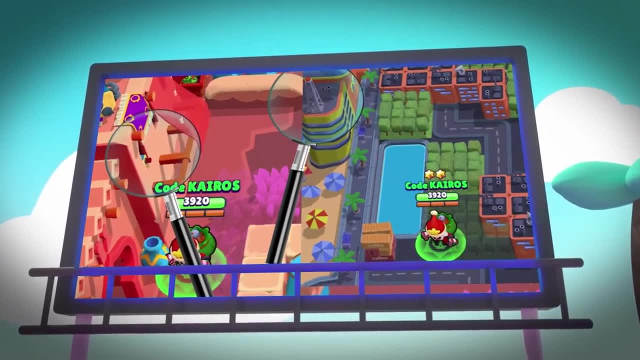 Ray even got a cease and desist order on the air. I was getting to that. You see there are blinking lights within certain Brawl Stars maps like Tara's Bazaar and the city level. When studied closely, they spell out a message in Morse code: WKBRL, the name of the YouTube. 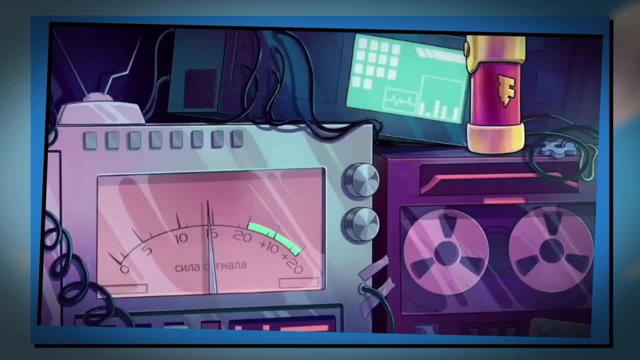 channel and live stream that Kyra and I created. The live streams start off as a source of cryptic information about future Brawl Stars updates. Nothing too exciting until one day everything changed. The broadcast was hijacked. Hello, Hi, Hey, I don't have much time. 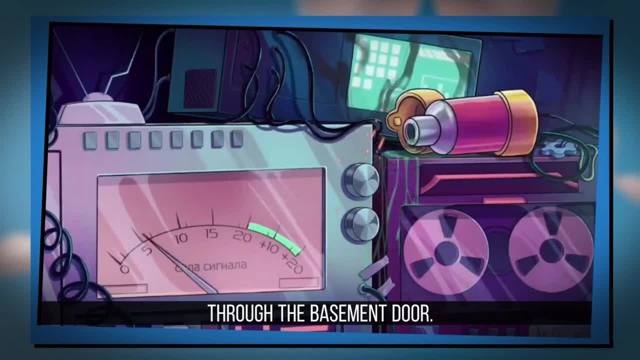 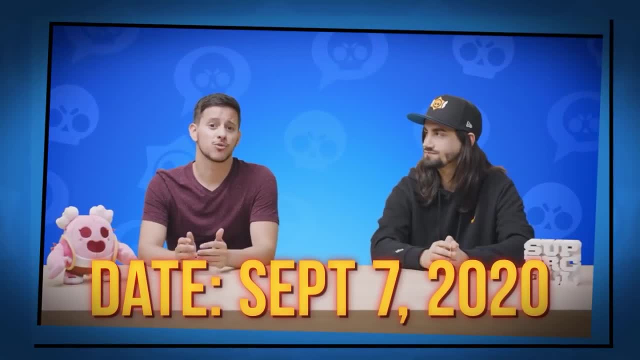 I snuck in here and I was able to dig in through the basement door. I gotta talk to you right now about what's really going on in this world. But the biggest reveal was yet to come. Two days later, interrupting the middle of an otherwise normal live stream, we get a. 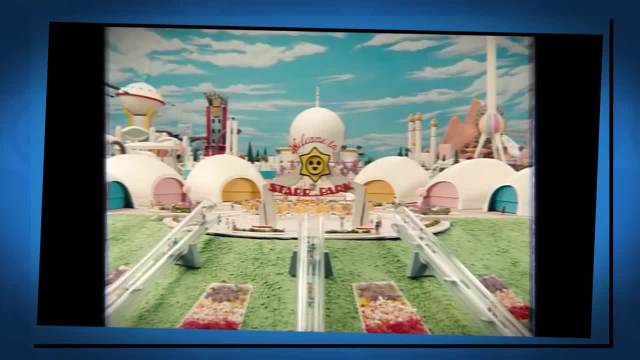 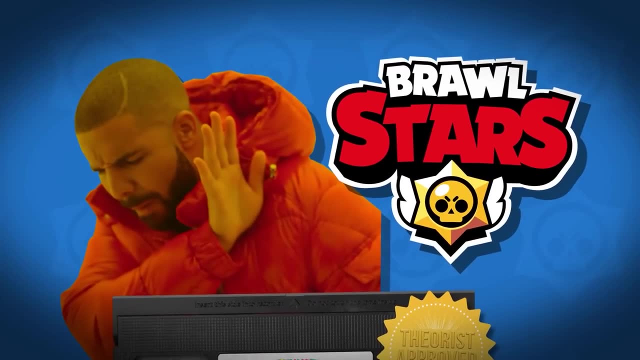 video that looks like an old VHS tape, created at a time when Star Park was looking for investors. Now this video is brilliant. It is a sight to behold, Like, even if you're not interested in this game or its lore at all. this six minute video. 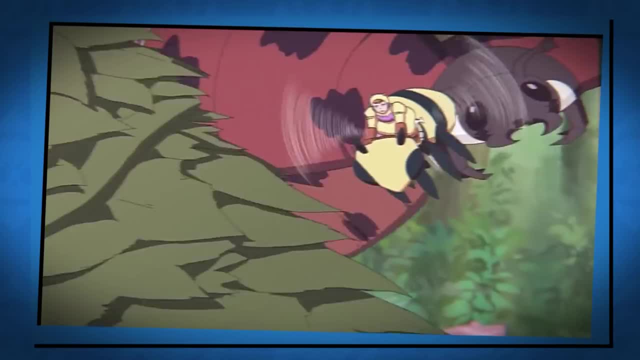 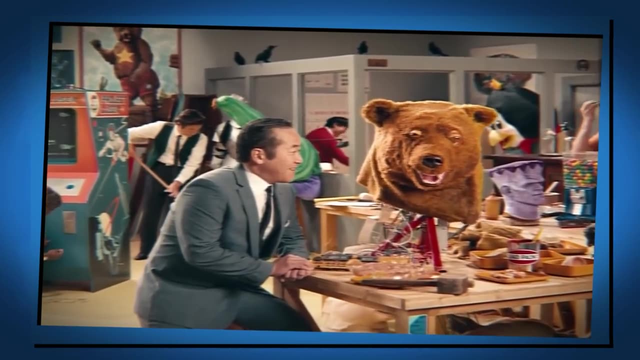 is just an incredible feat of production, with massive dance numbers, huge anime sequences, even rides Have a nice trip. Oh yeah, and there's also the scariest animatronic bear that you'll ever see, Dear FNAF movie. hire whoever made this video and threw it all. 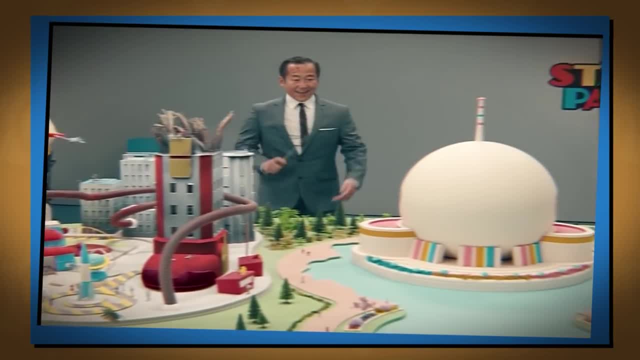 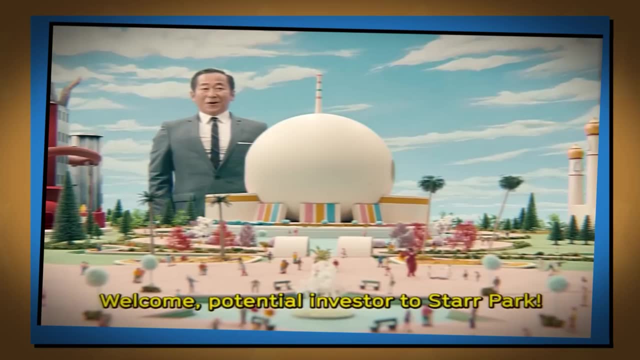 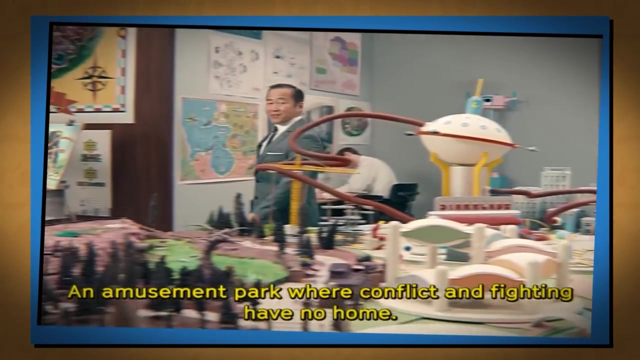 Buried inside these six minutes of insanity is more lore than you can shake an oversized pointer at. The video starts off innocently enough with a Japanese host inviting people to learn about an exciting new business venture. That's an oddly specific denial that you bring up there. 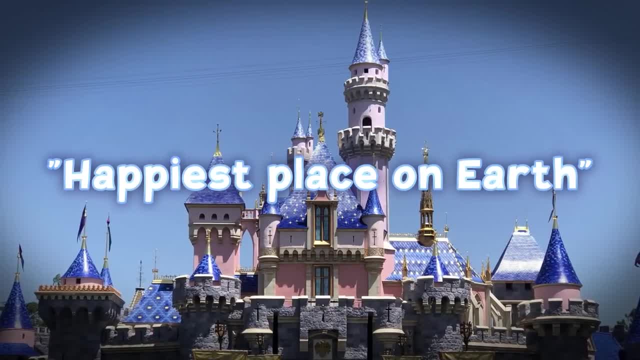 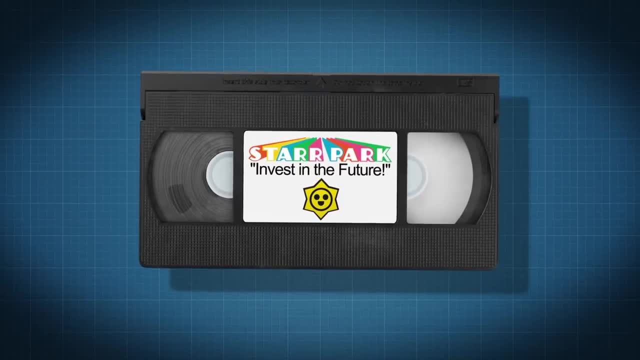 Look, I'm just saying that, as weird as happiest place on earth might be as a tagline, it would be weirder if Disneyland advertised itself by telling you absolutely no violence happening inside this theme park. Anyway, it appears that at the time this video was recorded, the park was still under. 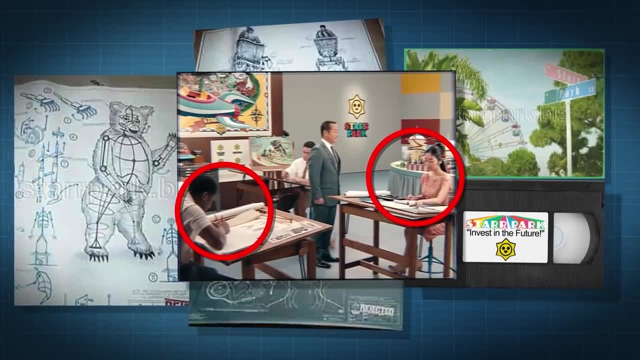 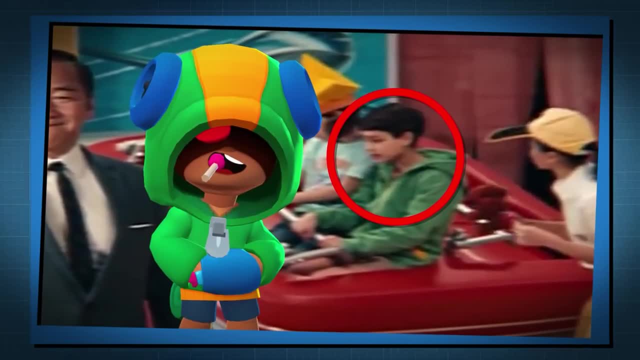 construction. Many of the rides are still in prototype and planning phases, but sprinkled throughout are references to characters and moments from the actual game, Like here: we have a young boy with a green hoodie that looks similar to the brawler Leon. 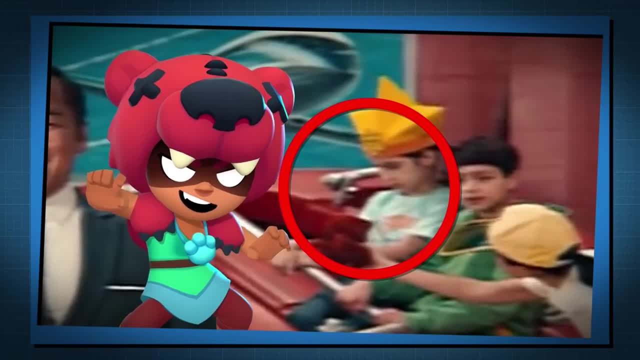 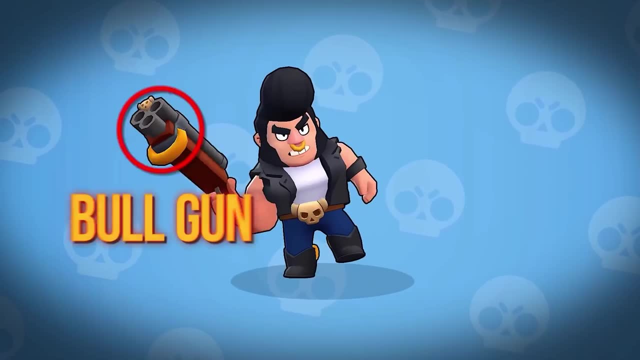 And the girl next to him with a teddy bear is just like the one that another brawler, Nita, uses during her super. Did you know that those two are actually confirmed siblings? Yes, Yes, I did. There's even some recognizable firearms in the form of the bull gun. 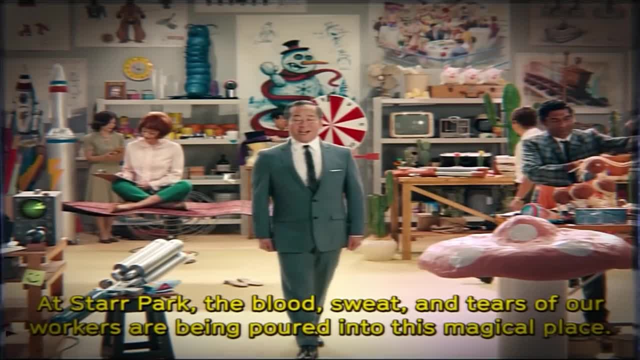 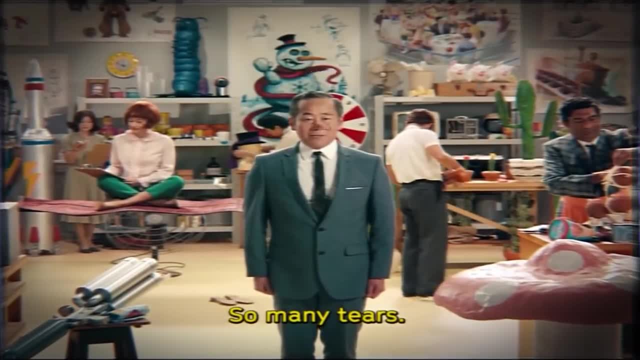 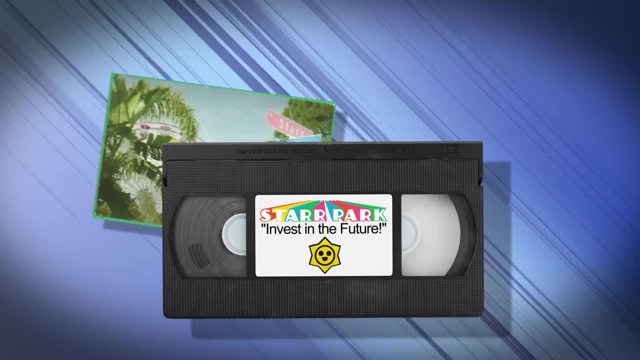 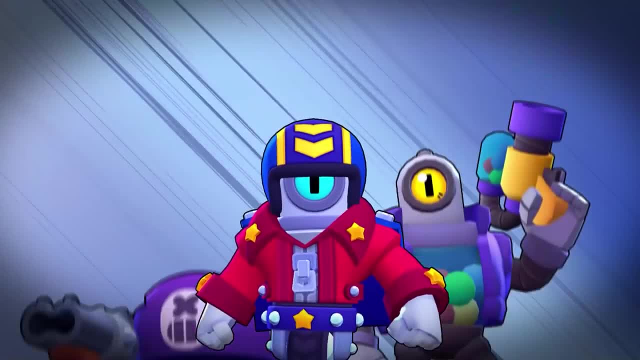 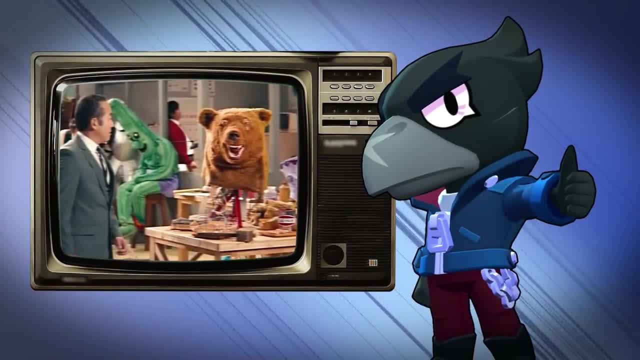 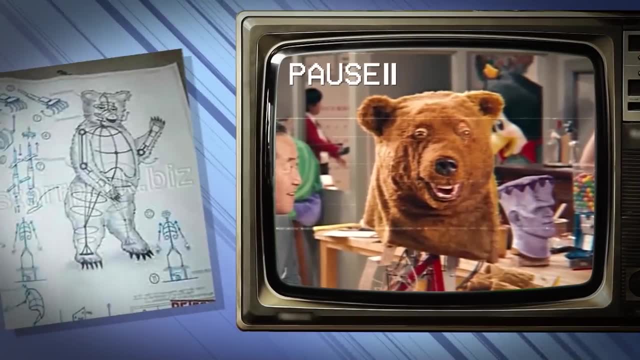 Why are some brawlers like crow bipedal animals? Well, we clearly see animatronic animal heads as a real part of this park, More real than anything you can imagine, Which, by the way, also has schematics posted to the StarParkbiz website. 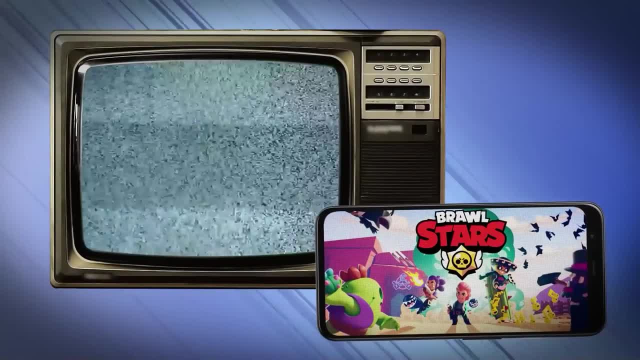 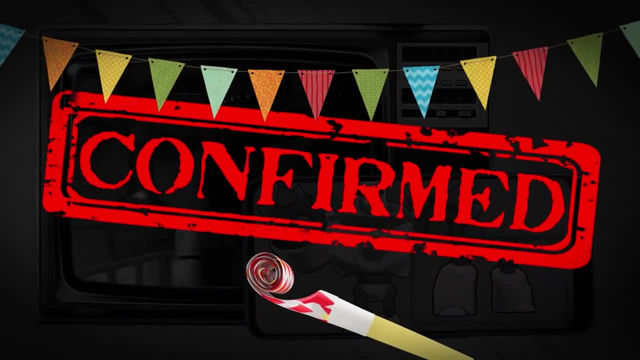 We even see what appears to be the origin for several fictional characters within the Brawl Stars universe, like in this shot, which shows what looks to be the giant boss robot from the game. So, theory confirmed, right? Well, yes, but also no Towards the end. 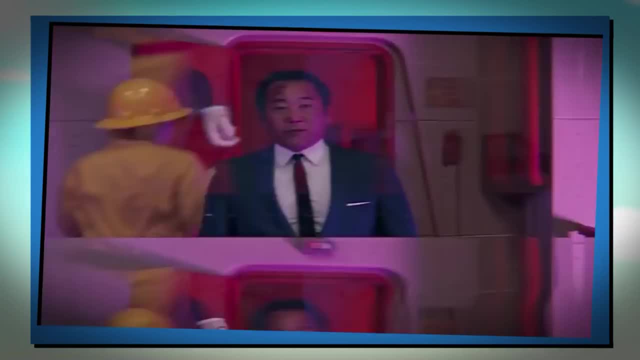 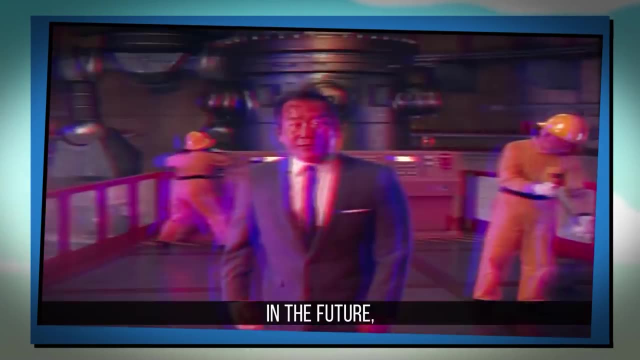 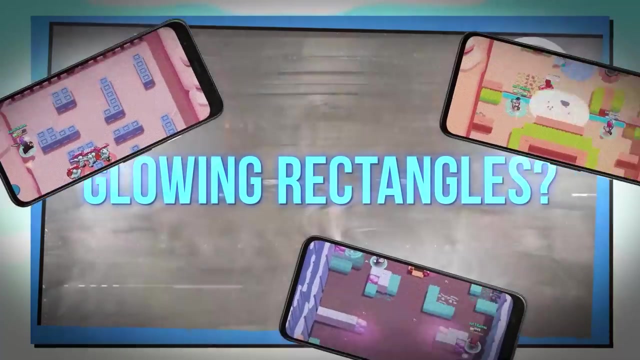 everything seems to break down and we hear what's clearly a backwards message Which, when reversed, says this: Glowing rectangles. What could that be referring to? It's this MadPat Glowing rectangles. This is how we control them. 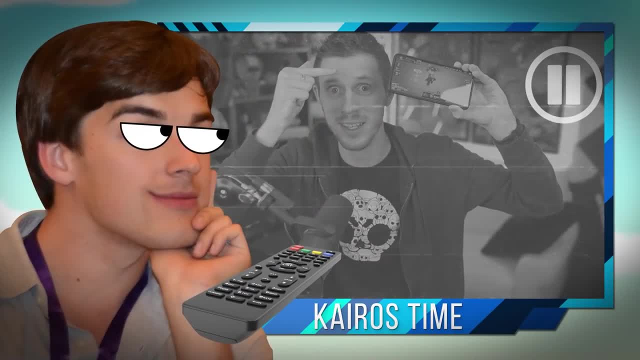 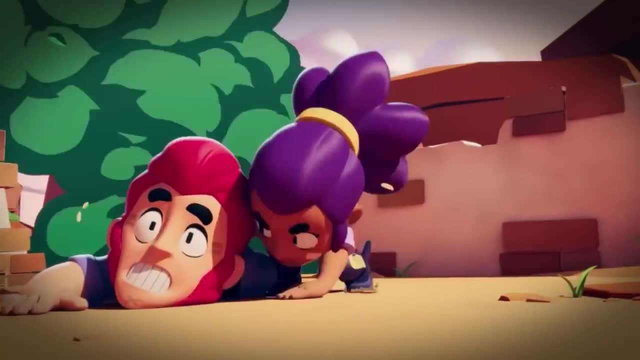 Yes, Kind of a rhetorical question, but I appreciate the enthusiasm. Obviously, this message is referring to us controlling the brawlers with our phones, Children of the future with glowing rectangles. So those brawlers that seem all too eager to shoot each other in disputes over gems. 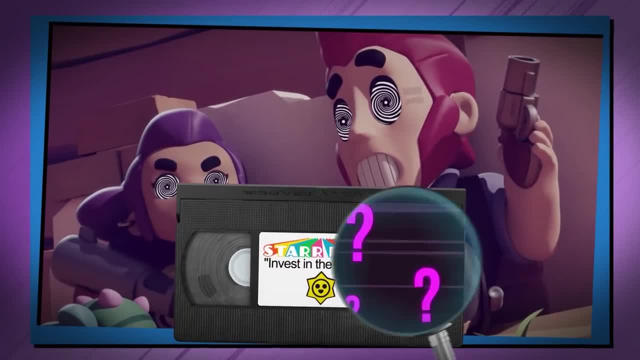 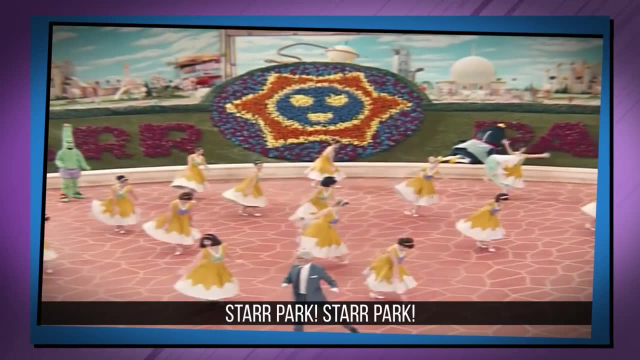 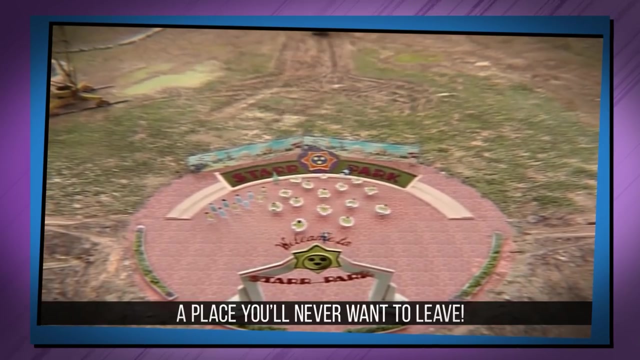 it turns out, aren't doing it on their own accord, Which also explains some other hidden message That happen when you play the video backwards. In the original video, we close out on a bunch of dancers as we hear the song, But backwards suddenly, this outro becomes the first thing we hear and, um, the message changes a little bit. Listen for yourself. 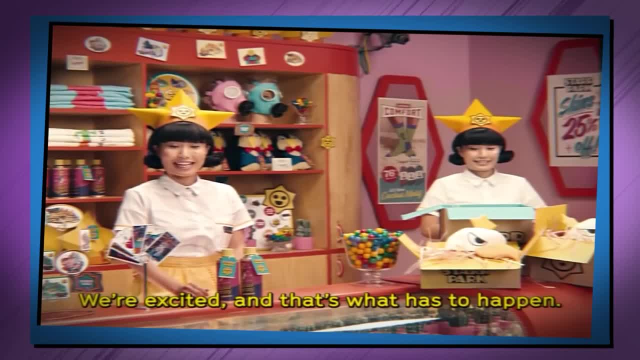 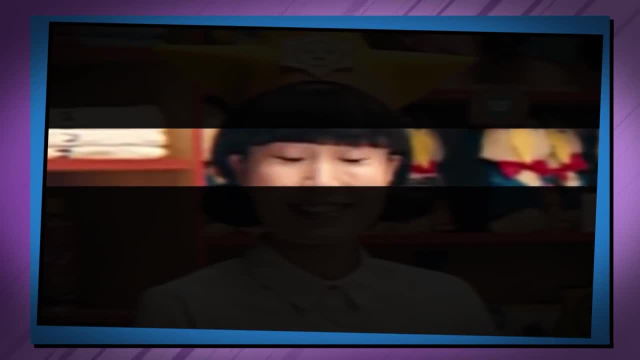 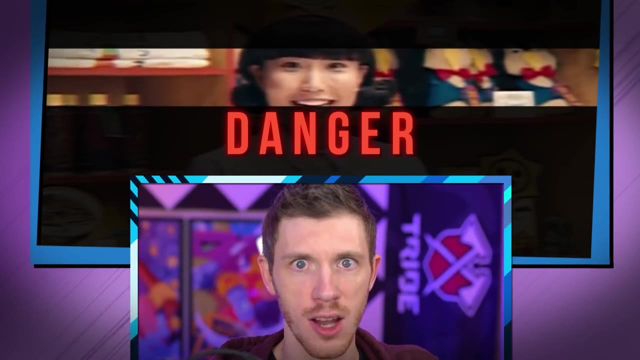 Or what about this clip? Did you catch that? Not the smile, Not the spoken dialogue, but the woman's erratic blinking. She's blinking in Morse code and it spells out Danger, It spells danger. D-A-N-G-E-R. 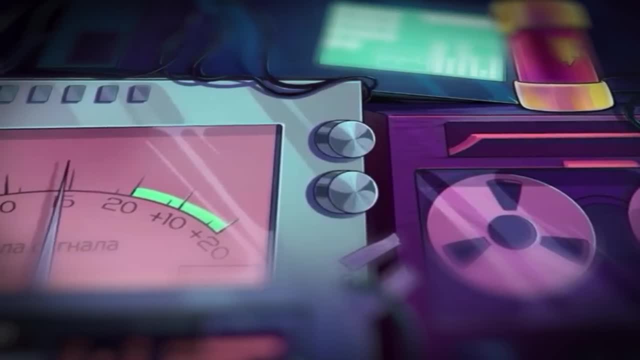 Th-thank you, Kairos. And now it's probably time to explain how the WKBRL stream fits into all this. Earlier this year, the WKBRL channel rebranded as WKBRL- The Voice That Hears You. 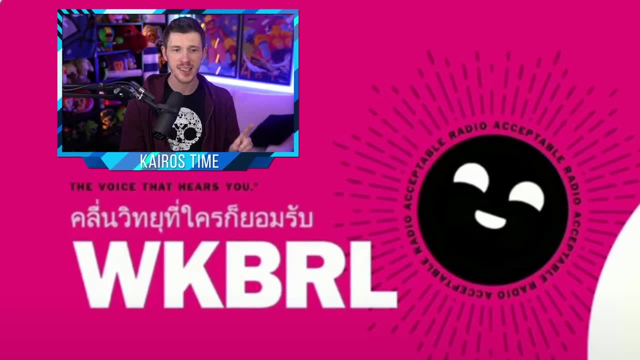 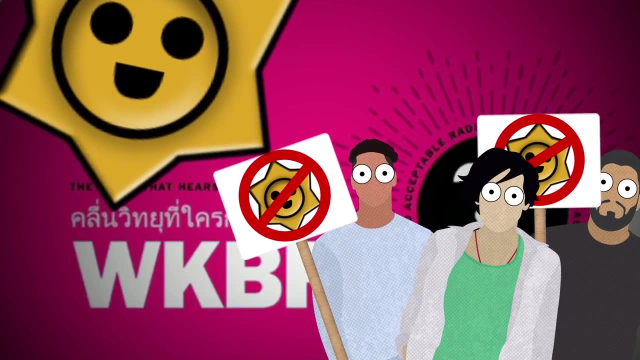 Well, not so much rebranded as taken over. The current theory is that the WKBRL network used to be run by a renegade organization trying to fight back against Star Park, But when Star Park found it, they co-opted it to play a day-long loop. 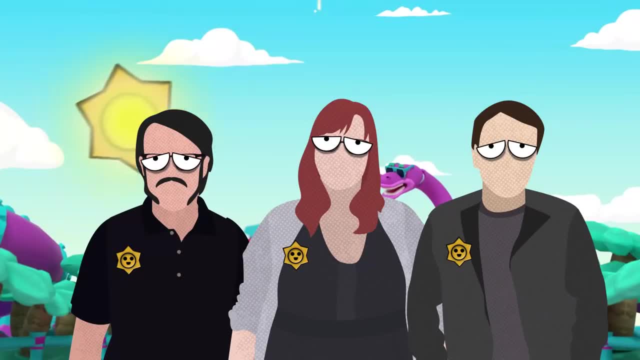 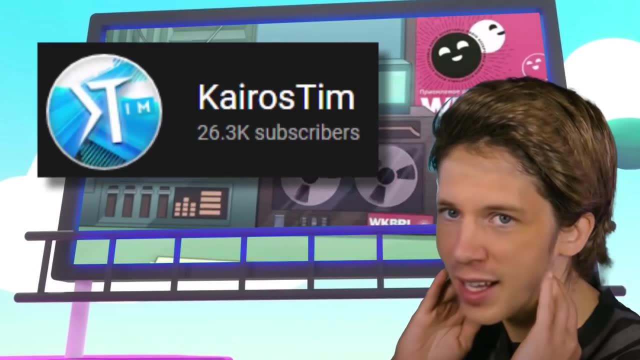 that seemed to be taking employees of Star Park through a 24-hour cycle forcing them to constantly repeat the same day, Starting with a morning workout by a fake Kairos named Kairos Tim. Welcome everyone, This is Kairos and we're gonna work out. 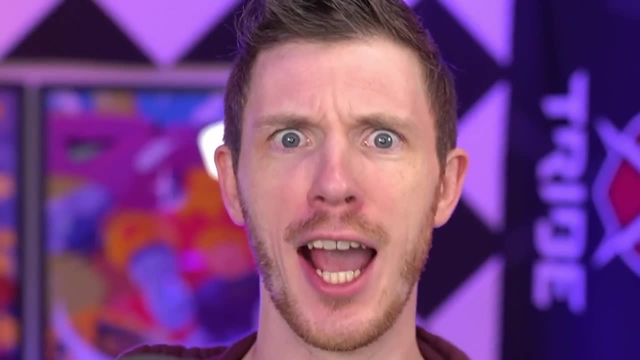 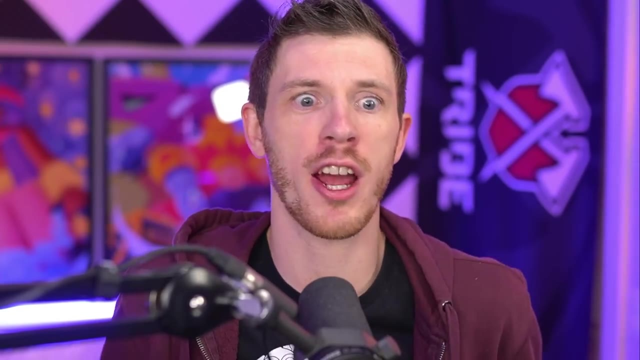 Hey, that's- that's you. He sounds nothing like me and he's clearly a fake Kairos. But this theme of keeping dissenters quiet, it continues. My channel is one of the main outlets for brawl theories, and I'm actually trying to spread the truth about what's going on. 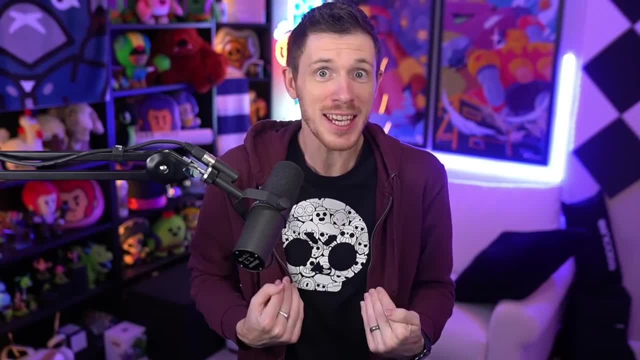 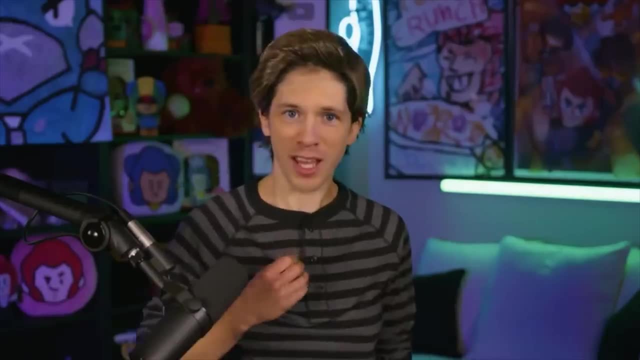 So how do they fight back? They try to discredit me with a fake Kairos, Literally a deep fake. Hello, fellow brawlers and welcome to Kairos. Tim With me, Kairos, Follow me. I'm the real Kairos, not fake Kairos. 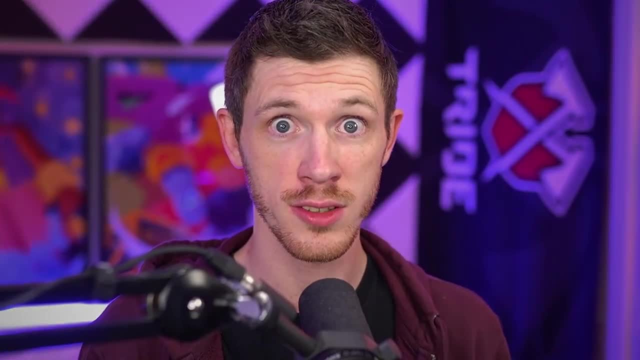 Then how do I know that you're you? You don't, Except that you actually do, because I can touch my face. Wait, what You're- you're supposed to be able to- Touch your face, I'm just a cutout. 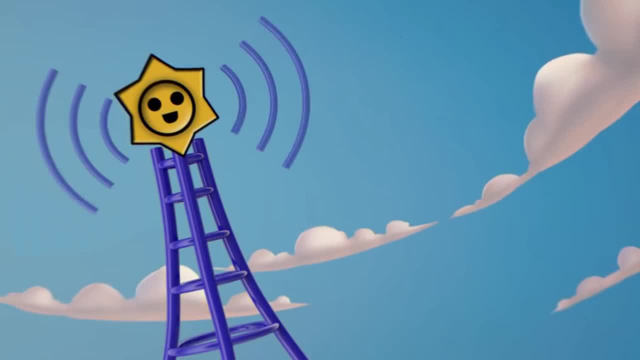 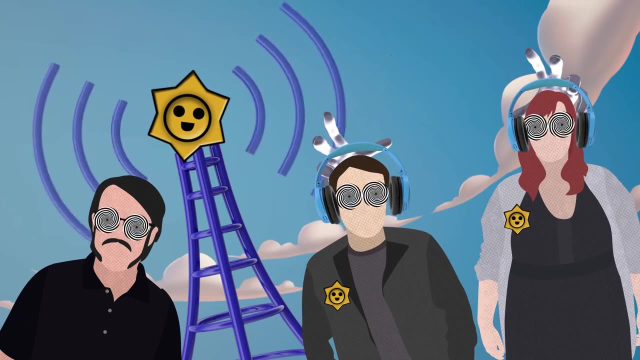 I- I can't- Oh, Oh, phew, that was close. Anyway, their broadcasts have a constant theme of brainwashing. almost like Star Park, employees are being forced to listen to this every day to ensure that they obey their programming. 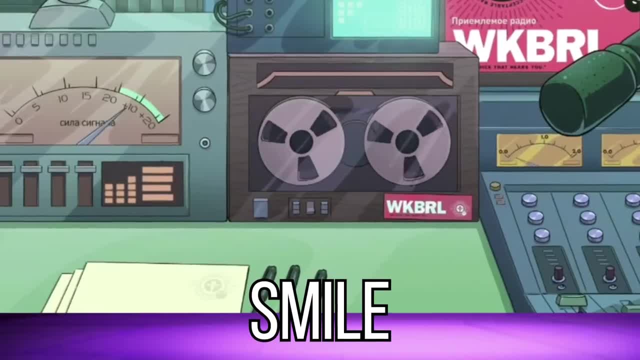 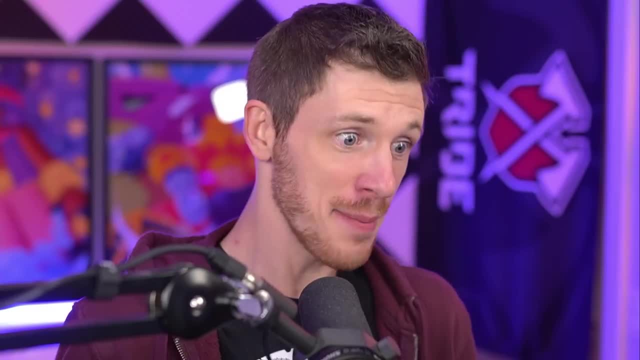 This is your smile reminder: Smile, Smile, Smile And fake. Kairos is constantly mentioning that you don't have to worry about being turned into a brawler. Kind of makes me think that they're turning people into brawlers. So we have people being kept here against their will. 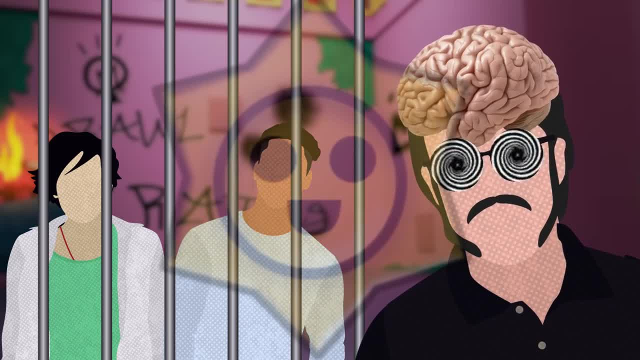 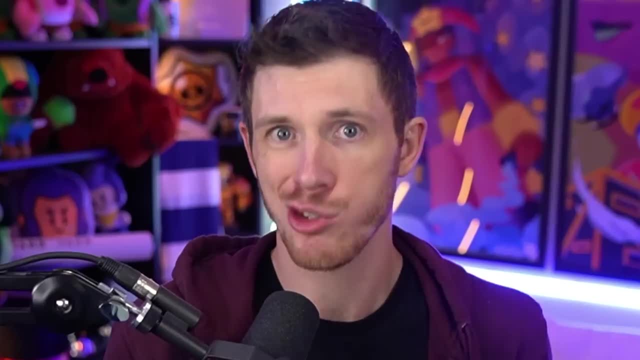 as well as themes of brainwashing And being kept under the control of others, all to turn humans into fighting warriors, Exactly. And we also get constant hints that the people being brainwashed in Star Park are actually asleep. If you're experiencing awakenings, 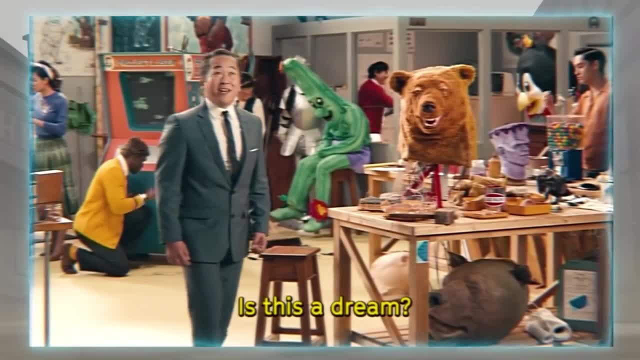 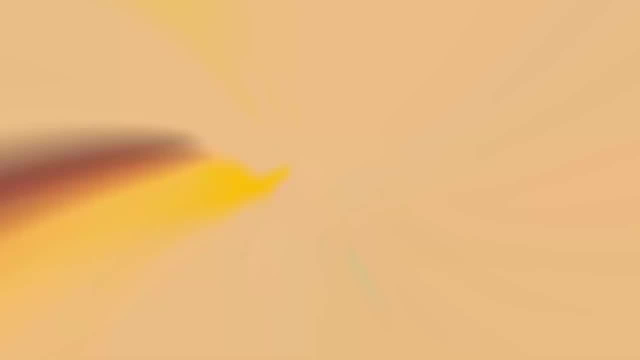 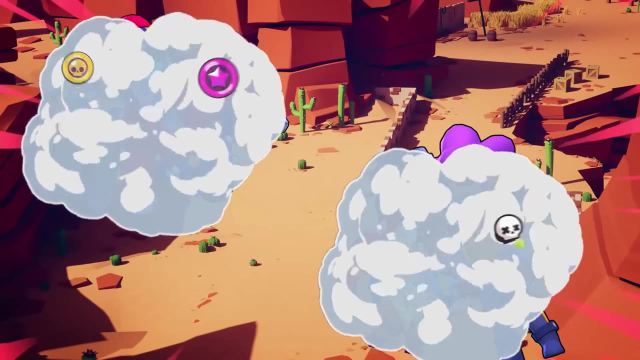 don't, Just don't. Nope, it's real, And this confirms my theory that all brawlers are forced to do battle all day, every day, in a simulated dream world. Hold up, You don't seriously think that they went with the? 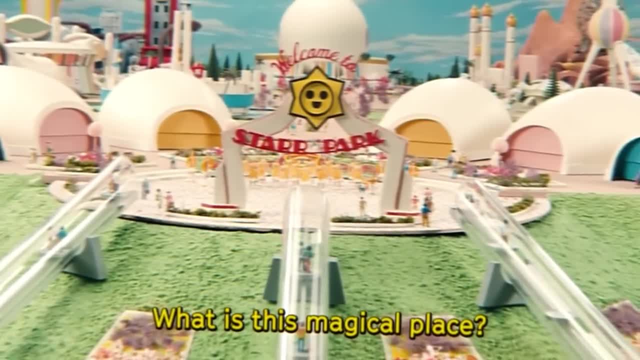 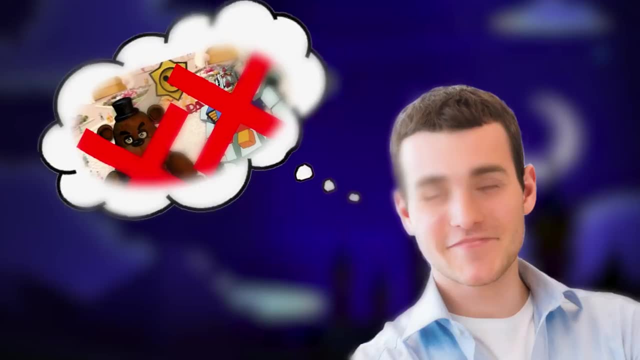 It was a dream the whole time? shtick, do ya? If that were true, why would they need an elaborate real park? Why would they build animatronics and giant mechs? There's no need for all of that if this is just a dream or happening inside the mind-scape. 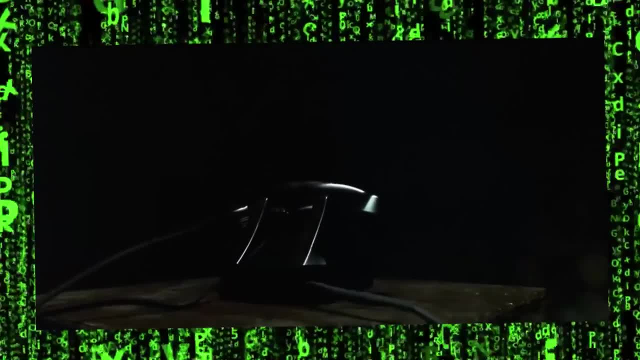 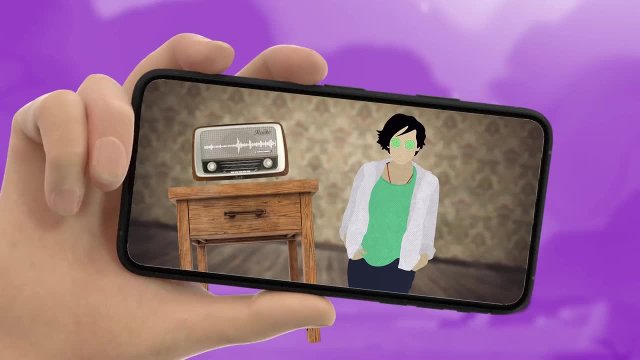 No, I would argue that it's more like everyone's caught in a trance-like state, Kind of like the Matrix, you know. Their conscious mind is asleep, being distracted with these daily activities that we hear on the radio, while their bodies are being controlled by us. 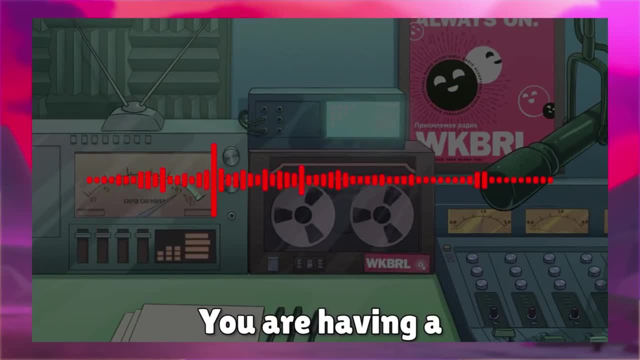 That's why the radio simultaneously tells the listener to wake up and also go back to sleep. If you are awake, you should go to sleep, Go to sleep, Sleep. It's placating the minds of these people so they don't realize what's really happening to their bodies. 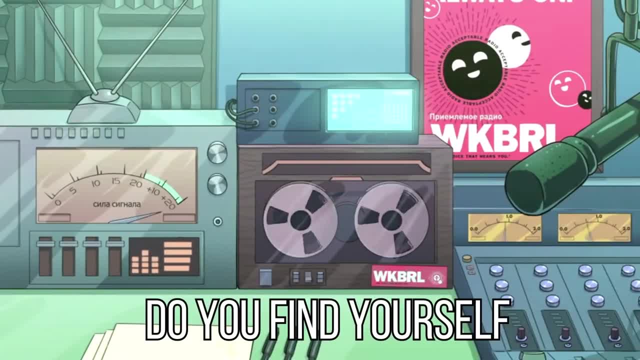 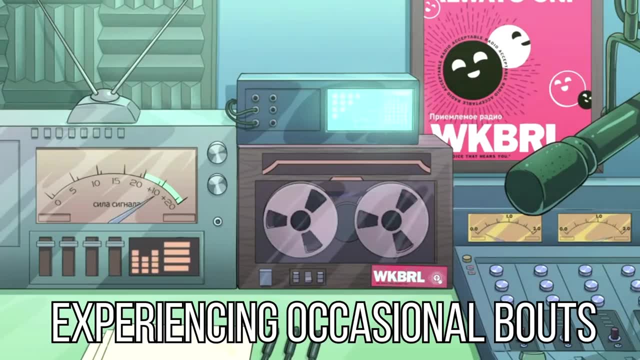 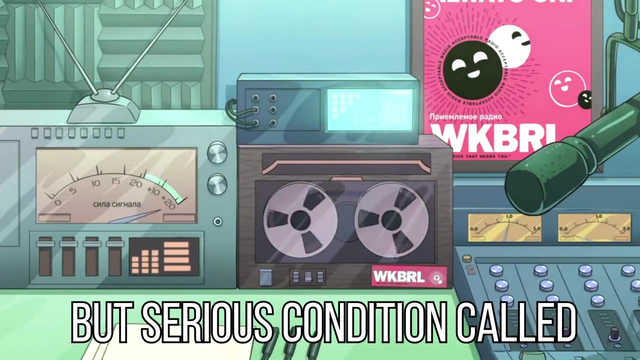 Listen to the way that these videos describe awakenings. Do you find yourself questioning your station in life, Having flashes of another plane of existence, Experiencing occasional bouts of sudden realness? If you're suffering from these things or more, you may be experiencing a rare but serious condition called awakenings. 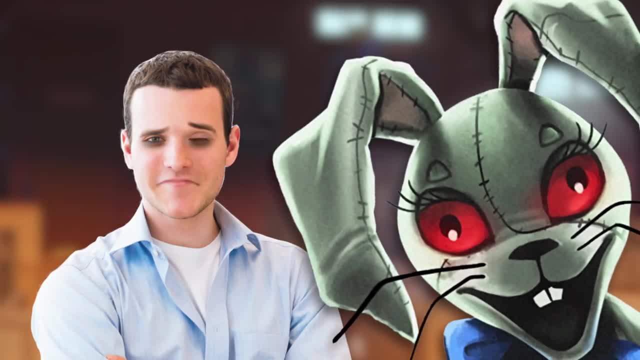 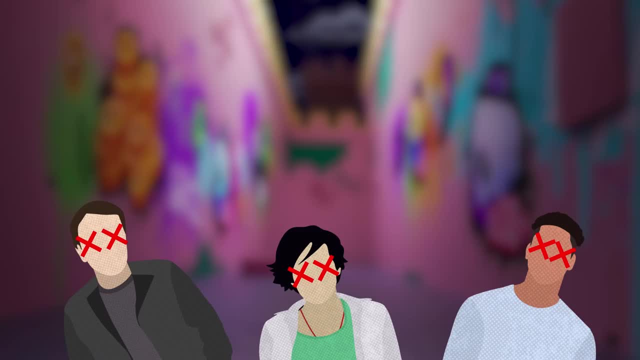 It doesn't sound like a person waking up from a long nap. Sounds more like a person who's coming out of a trance and realizing that their mind has been trapped inside of a body that's being puppeteered by another person. But that doesn't explain how everyone's able to endlessly respawn. 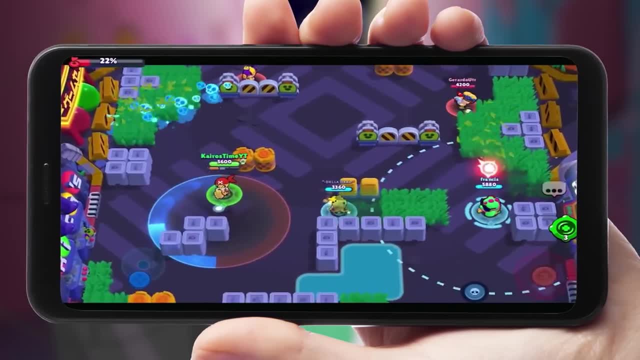 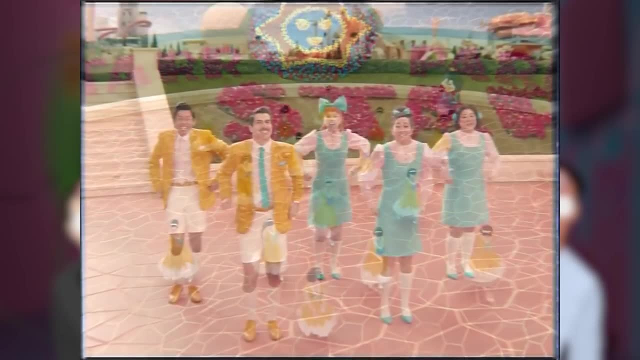 If you get shot in real life, you're not getting up to fight another day and you aren't going to be able to participate in hundreds or thousands of battles, Whereas if it were in a dream, then you actually could. But then why the need for a physical park? 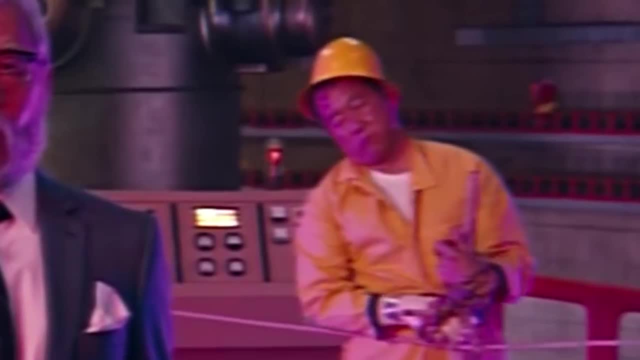 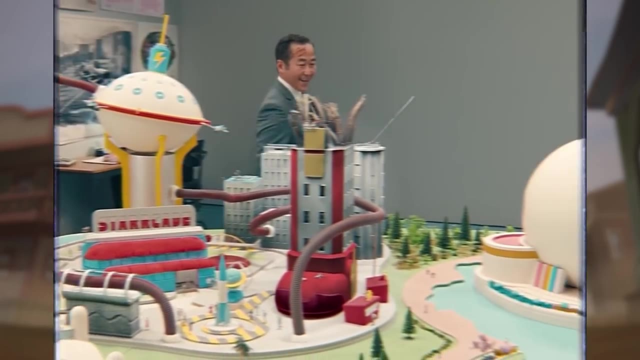 And why would people in the Investor video be walking around with their eyes closed? Well, what if we're both right? Maybe there are layers to the simulation? okay, This part of the Investor video always struck me as kind of odd. The presenter taps the model of the park with his pointer. 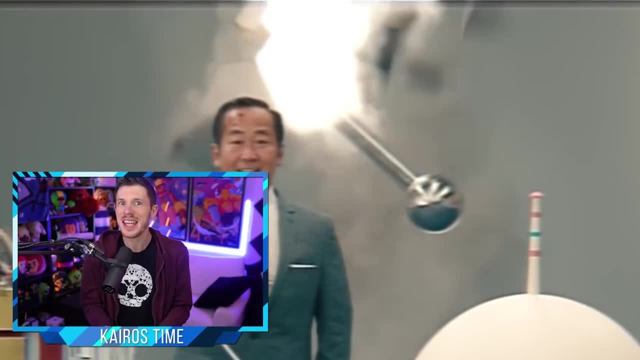 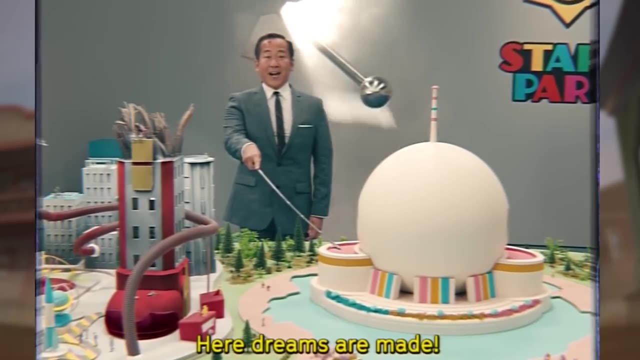 and you see a jumbo version of it appear behind him. It's almost like he's pointing at the model that he himself is in Kairos. you genius, I could kiss you. Uh, please don't. That clip shows that there's a physical connection between the model world and the physical one. 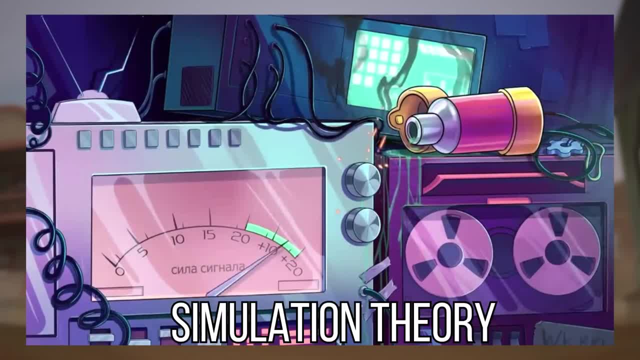 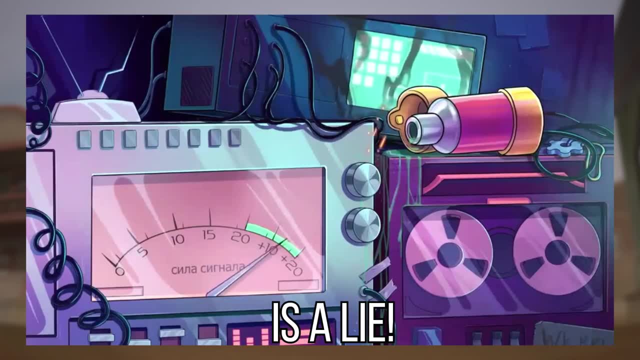 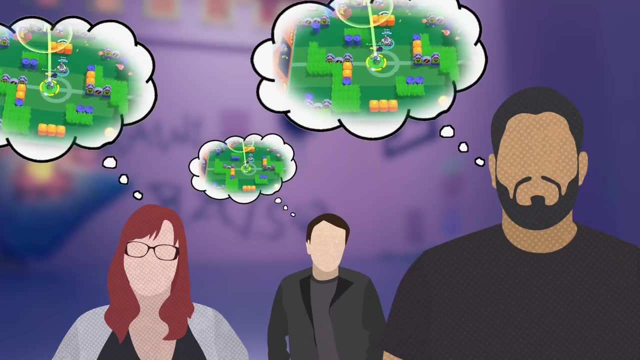 We also have many voice clips referring to simulated realities. You know about it, of course you do. But what if it's true? What if everything is a lie, everything illusion, and I am inside a simulation? What if these simulated realities are the dreams they have? 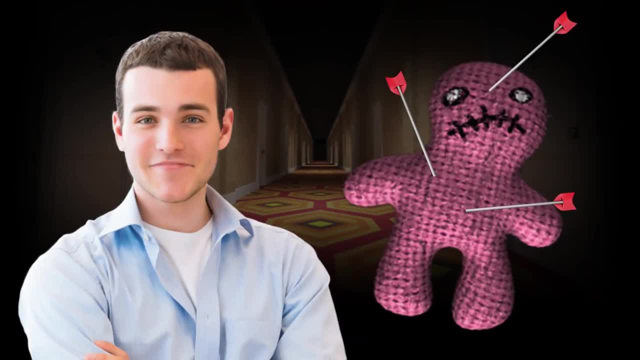 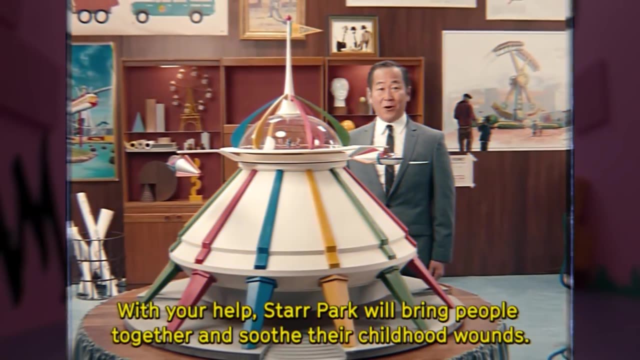 but they actually exist in physical form in these models Like a voodoo doll in reverse, Where the doll is a real person and the body is actually an empty vessel being controlled by somebody else. Think about it. In an earlier part of the clip we see the presenter lean over a glass case and say: 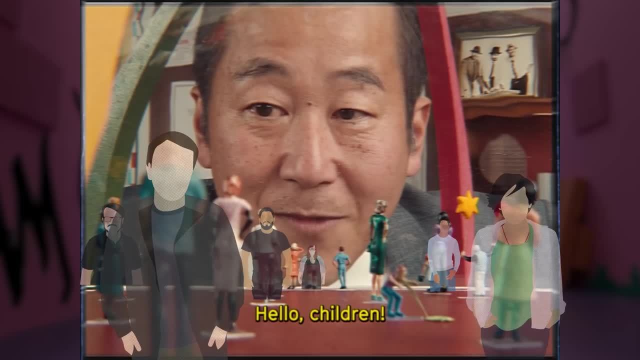 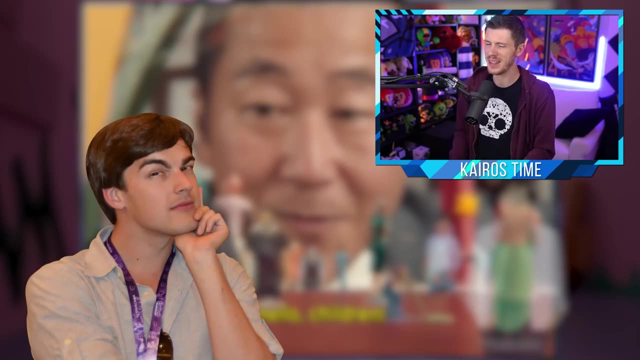 hello children. What if he's talking to real people, people whose consciousnesses are stuck inside the models? so you're telling me that the brawls are happening in a model park and not the real one precisely, but why do that? and that still doesn't. 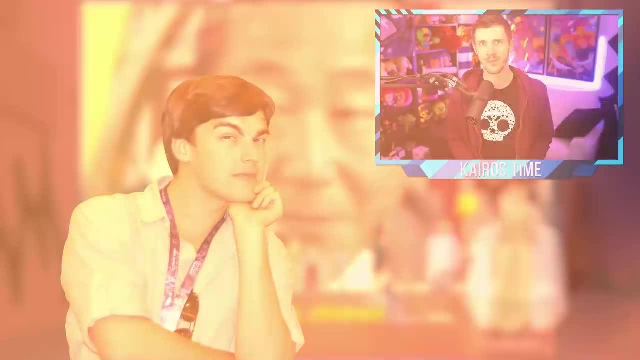 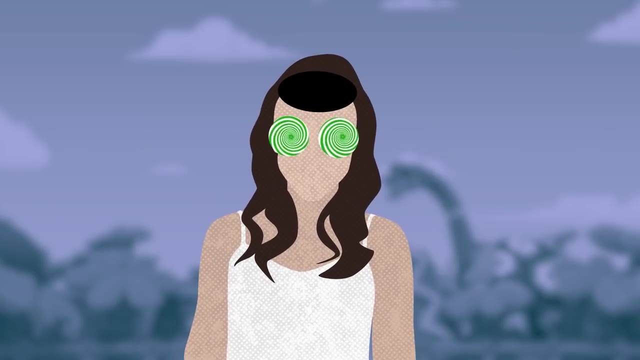 answer the actual physical park question. well, consider this. like you pointed out, they seem to need human minds to power the brawlers. but where do you get them? you divide the body and brain in two. on one side you have the real people in the real park that are kept in this trance-like. 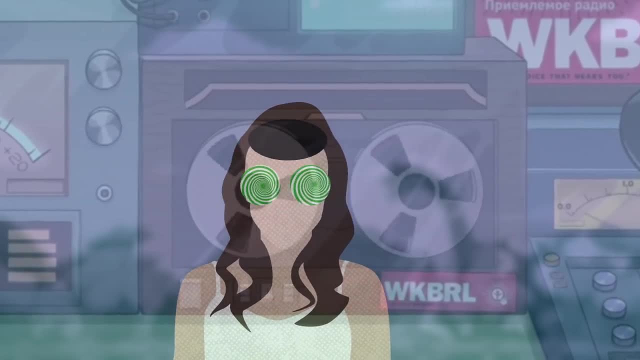 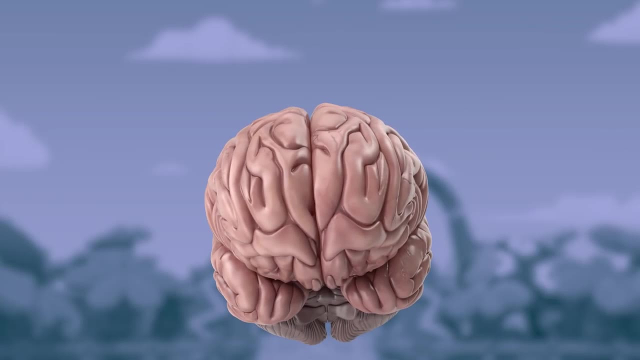 state. you hypnotize them with the wk brl stream so that they go through the daily motions: they eat, exercise, sleep, etc. that keeps their body happy, which leaves the rest of the brain, the higher processing power, to get funneled into those models, thereby creating or running the brawl stars. 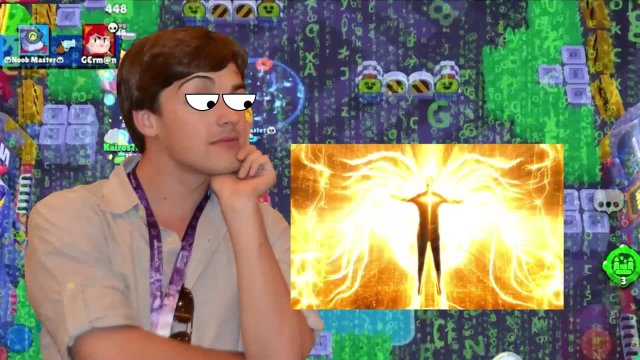 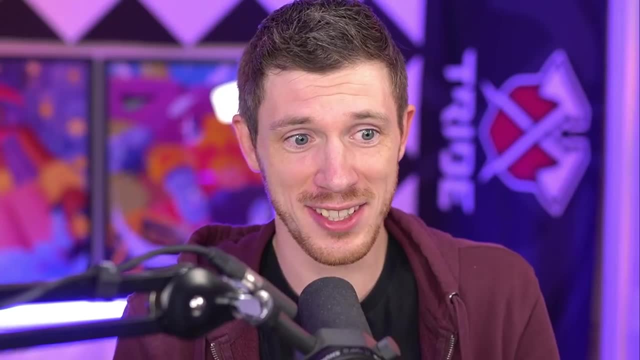 matches again. it's just like the matrix, except with a hundred percent less religious imagery. that does actually solve why they would need a real theme park and how the characters actually get respawned over and over, but honestly it leaves me kind of disappointed if all this is just a set. 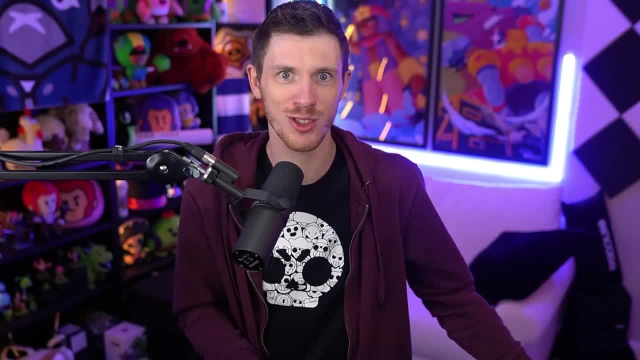 of toys battling. i feel like it kind of cheapens the whole mind control thing. we all used to make our toys fight as kids, but now they're fighting as kids and they're fighting as kids and they're fighting as kids and nothing bad came from it. why would they actually need real people? well, that. 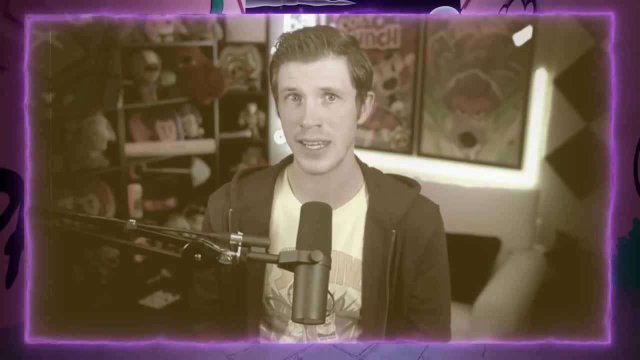 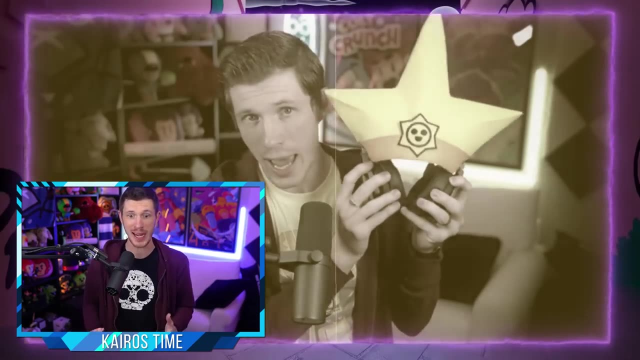 actually brings me back to one of your theories, that all of this is just star park preparing for world domination. yeah, one of my early theories was actually that all matches in brawl stars were battle simulations- trying to train up ai. what if it's not training up ai, but people? here's another. 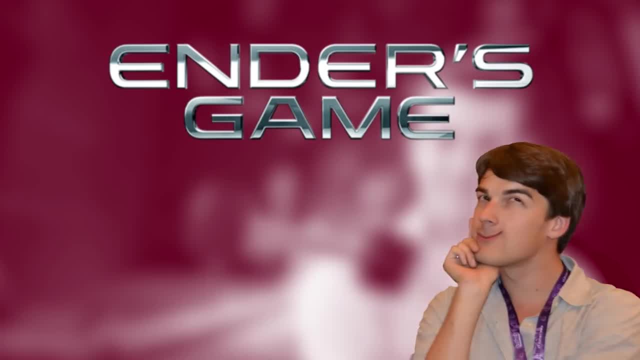 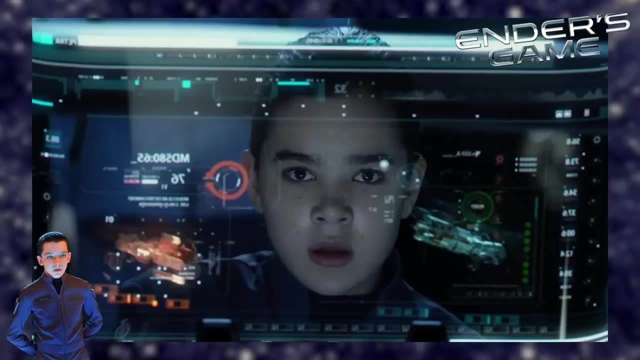 pop culture reference for you: ender's game. have you read it? i actually i'm about to spoil it for you anyway, so it doesn't matter. basically, it's about children playing through simulations to learn how to command star fleets in order to destroy an alien threat. but it's not just about 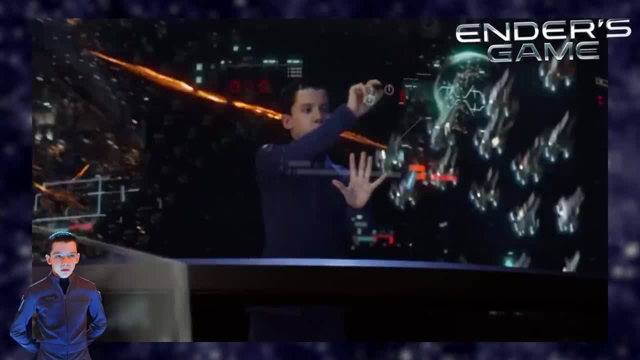 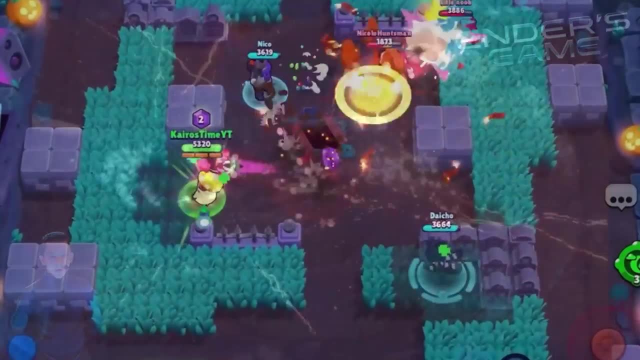 that it turns out what they think is just an exam was actually them commanding real ships with real people in a war zone. i'm proposing a similar idea. by having real people's consciousnesses trapped inside of the characters, they're learning tactics, survival skills and combat. look at leon and nita. 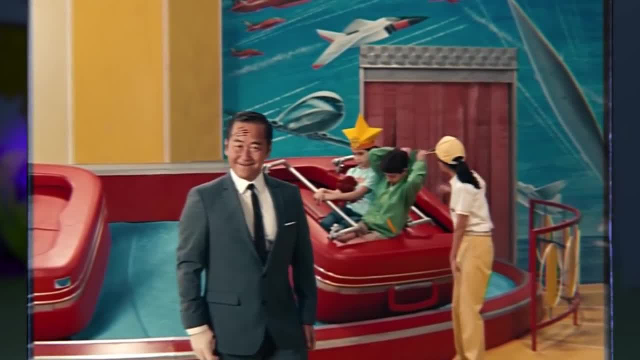 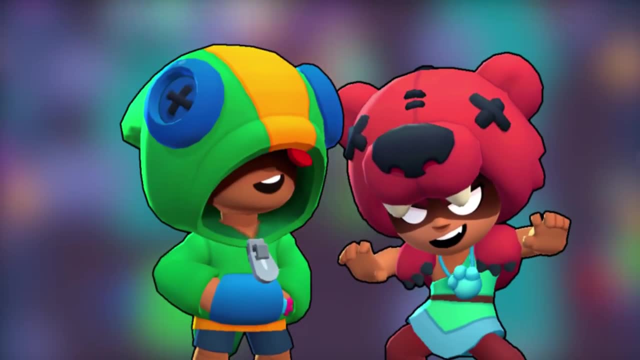 for example, two children that are going through the mindless daily wkbrl activities at the park, all while their conscious minds are connected to leon and nita to train them into super soldiers. their bodies are staying in peak health thanks to wkbrl pushing them through tough daily workouts. 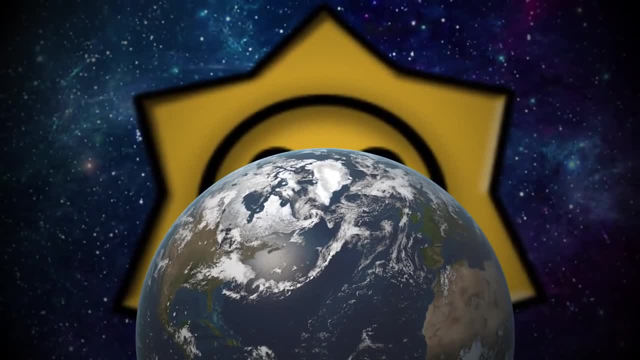 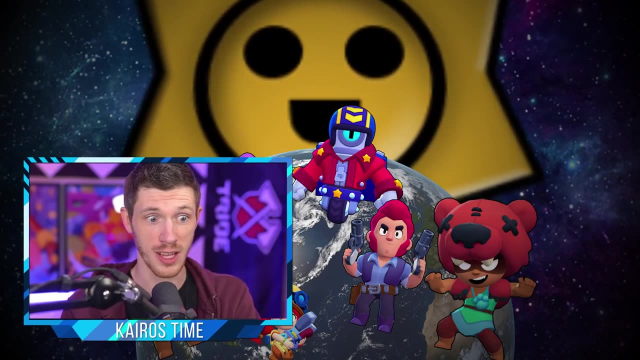 and their minds are constantly running training simulations. star park can activate this real life army of super soldiers to take over the world at any time they want, and we've been training them the entire time. so when do we get a new update? we don't know. somebody actually shut down the wkbr. 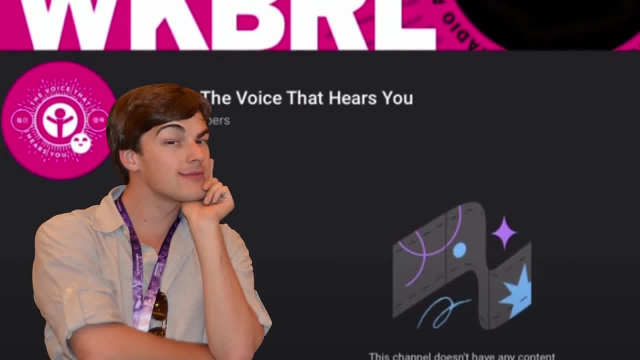 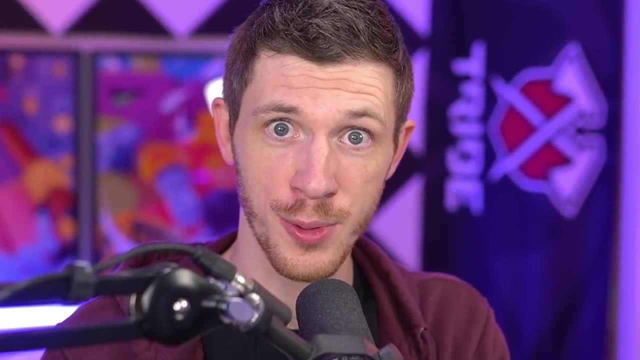 live stream just a bit ago and we still have no idea why. who knows, maybe this video will get their attention. we'll know if we're close. if you start getting deep fakes- core packages in the mail, just stay safe out there. star park is ruthless and welcome to the theory family wait, shouldn't i be? 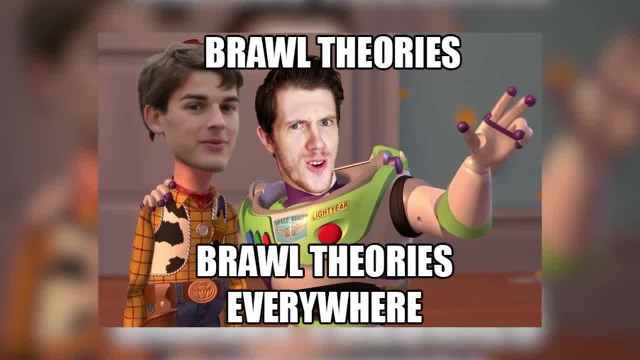 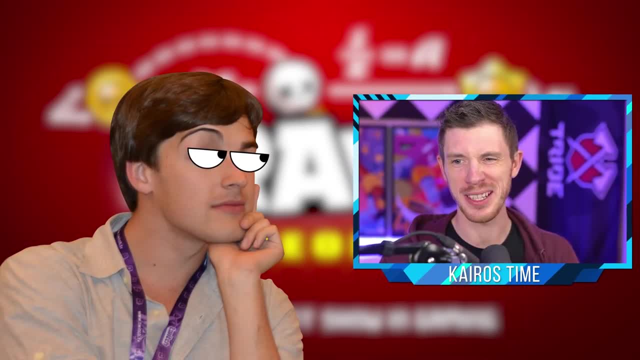 saying that to you. one thing we probably should say is: but hey, that's just a theory. theory. you just had to say it, didn't? you started as a joke, but it's kind of my thing now. trust me, i get it. and thanks again to kairos for being willing to listen to me stumble my way through. 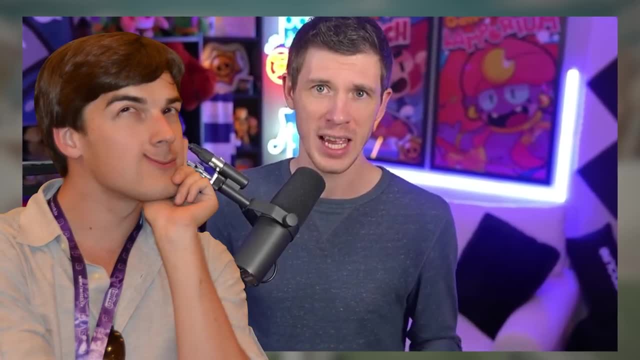 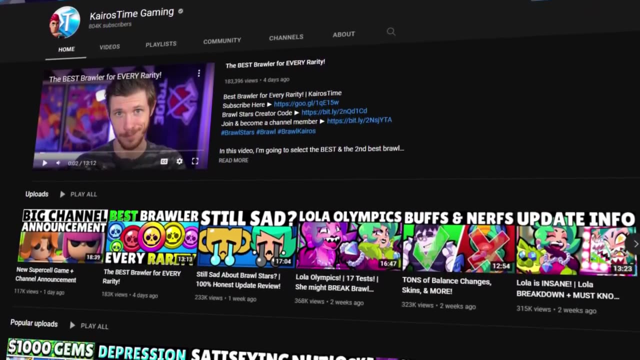 something that he knows way more about. there is so much more that would have been fun to talk about here, but then the video would have gotten really unfocused and bloated. so if you liked what i discussed here today, i highly recommend that you go over to kairos's channel. 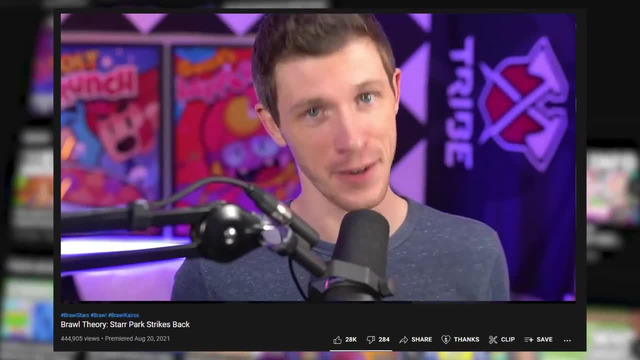 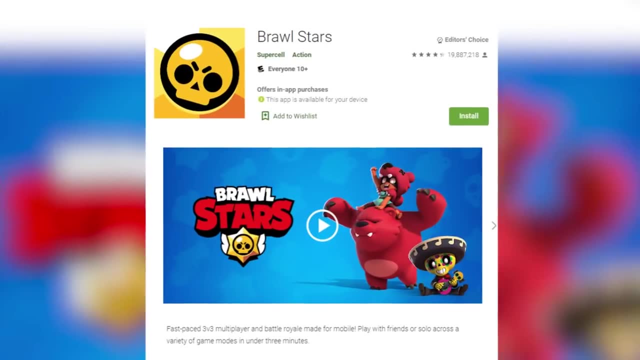 and take a look at his brawl theory series, where he breaks all of this down bit by bit, piece by piece, to lay out the entire lore of this thing. and again, it is still ongoing. we can have an update any day now, or, heck, you can just join the quest, pick up the game, take a look. 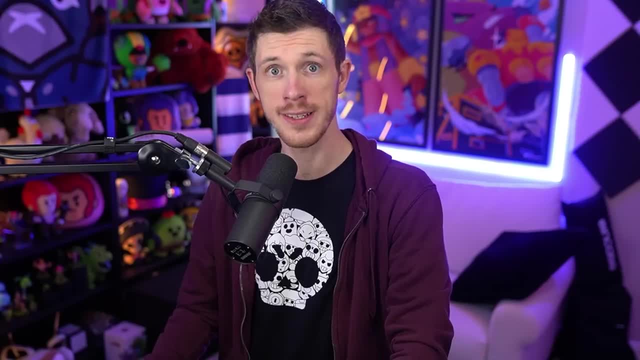 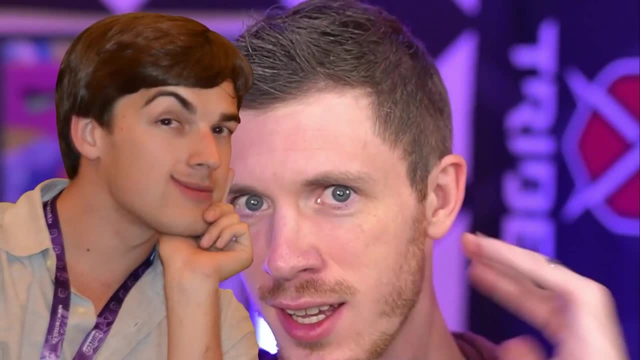 let me know what you find kairos. any last words before we wrap things up. yes, there is actually. i am the real kairos, and kairos tim is a fake and my hair is way more luscious than his. it's true, and nobody can deny that your dulcet tones and great audio quality are, in fact, the real deal. 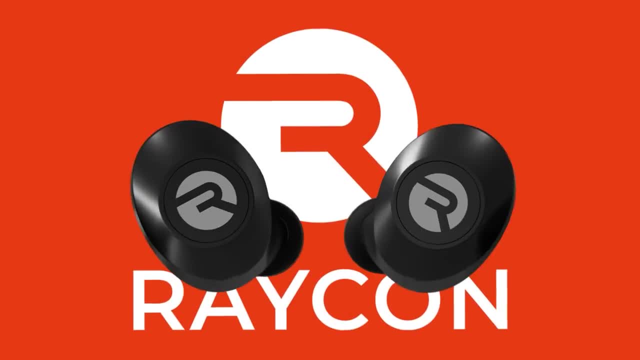 it's even more obvious when you're using today's sponsor, raycon wireless earbuds. hope you enjoyed the video, thanks for watching and i'll see you in the next video. Oh yeah, I am nailing those seamless transitions today. Seriously, Raycon's new everyday earbuds are phenomenal. 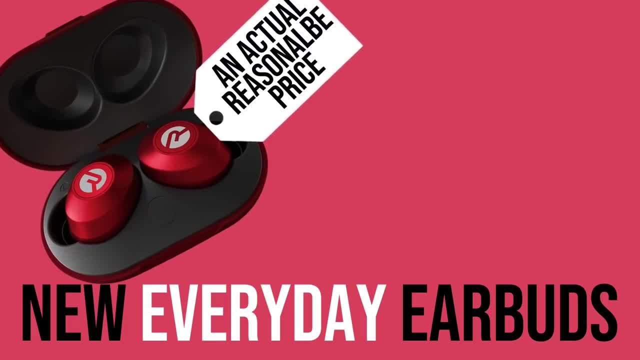 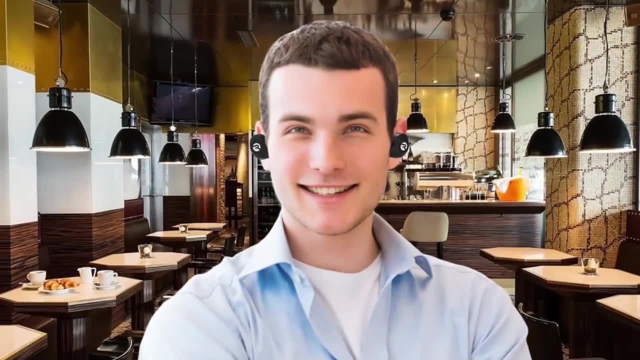 For just half the price of the premium brands, you're getting just as premium of an audio experience With Raycon. you're not throwing your money away on some hyped up and therefore marked up brand. Raycon is ensuring that you're getting the best audio quality at the best possible price. 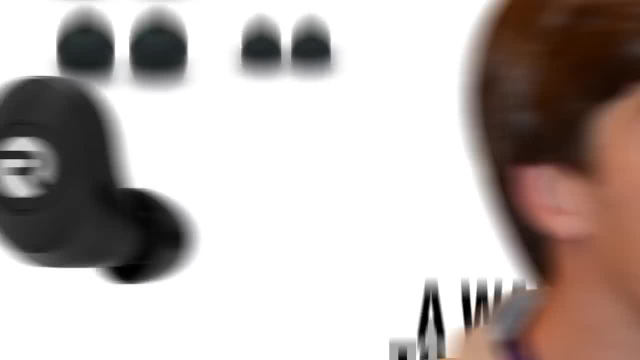 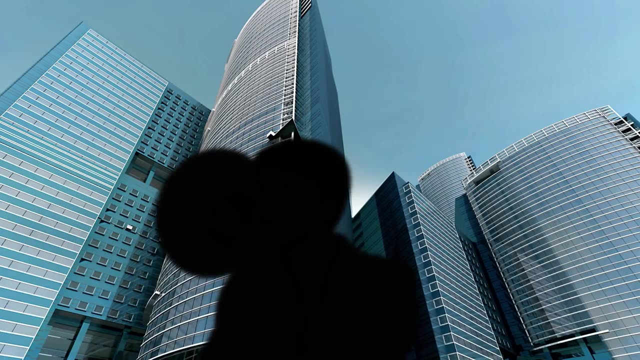 Raycon earbuds also come with a massive variety of gel tip sizes to guarantee the perfect fit for your individual ear. Dear other earbud manufacturers, one size does not fit all. Raycon understands that and gives you options to ensure a perfect fit every time. 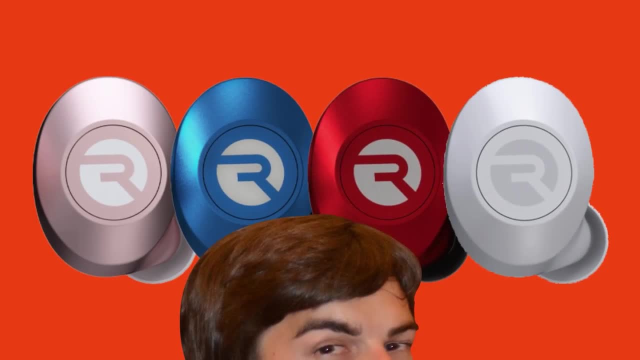 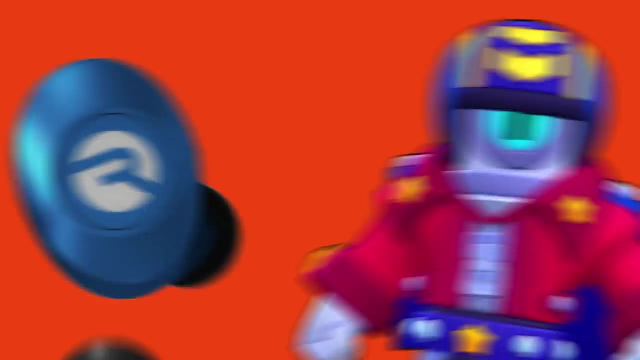 Raycon earbuds also come in fun colors Again, something else that the competitors seem to miss the memo on. With Raycon, you've got frost white, electric blue, rose gold, flare red and carbon black. You get the color that best represents you and your unique personality.